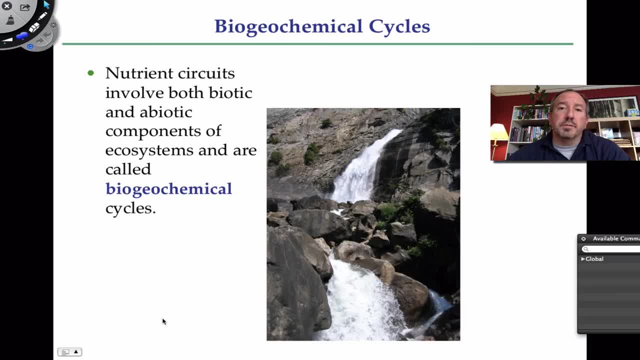 about, and so it's going to look at some of these crucial cycles. but one of the most crucial cycles, interestingly enough, is not necessarily a biogeochemical cycle in and of itself. it's simply the water cycle and, again, probably most of you are familiar with the water cycle. 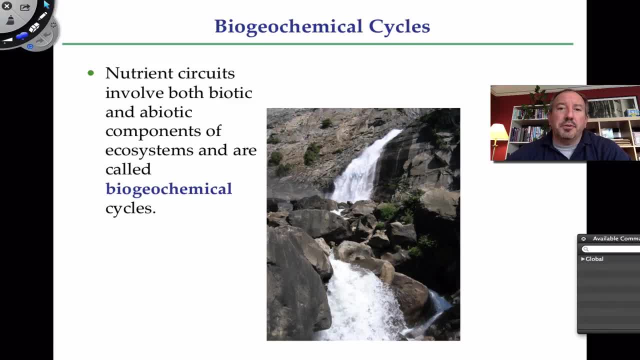 somewhere from your past, and so it has to do more with physical phenomena than it does with biological, and so let's talk about it. I put a picture here of one of the great waterfalls in Yosemite National Park, which is called Wapama Falls, and this enters into Hetch Hetchy Reservoir. 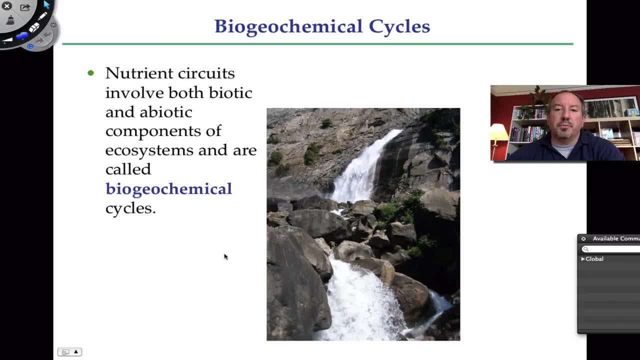 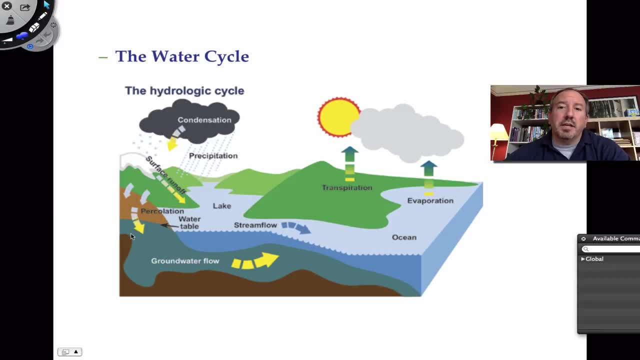 and so, as it turns out that this water that comes down from the side of the cliff is liquid water, and as it turns out, this water is liquid water, and it's not just liquid water, it's liquid water. this may be obvious, but liquid water is the state of water that I think is most usable when it comes. 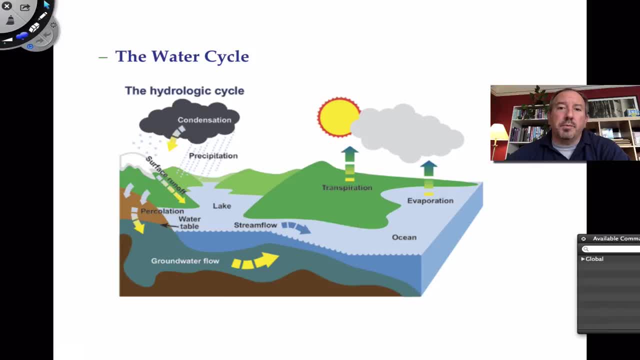 to biology. What are the other states? Well, you can have steam, you can have vapor, you could have frozen water, which is ice, and those are not necessarily accessible to biological organisms. and so let's talk about this water cycle a little bit. Due to the heat of the sun, radiation comes. 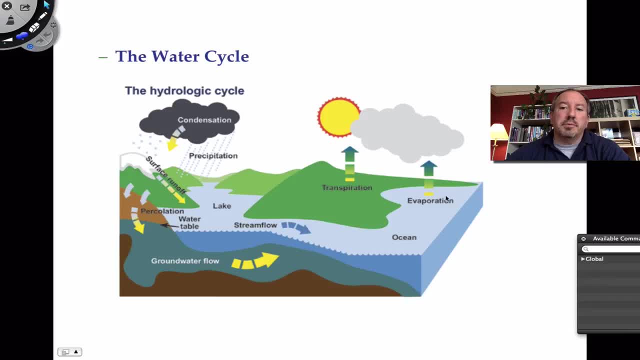 down and that infrared radiation comes down. and that infrared radiation comes down and that infrared causes the temperature to increase in the, in the water and warmer water, molecules will evaporate and travel up into the sky. Now this is a marine environment, so the solute of salt remains. 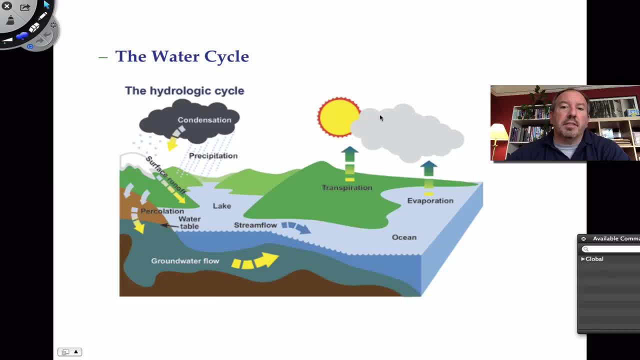 behind. so this is fresh water that's evaporating and then it condenses into clouds, and oftentimes those clouds will through the source of fog and wind, will come across and it will condense, and then, ultimately, weather conditions will change and then it will condense, and then it will condense. 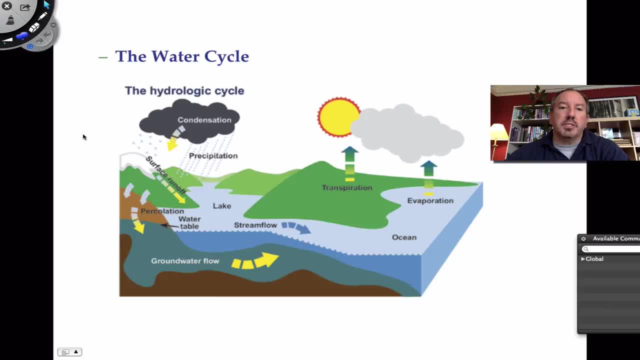 will cause. cooler weather conditions can cause precipitation. in other words, the rain will come down, and if it's raining on the land, this is fresh water, and so it's either going to run off the side of the mountain or it's going to collect in these reservoirs that we like to call these sink basins. 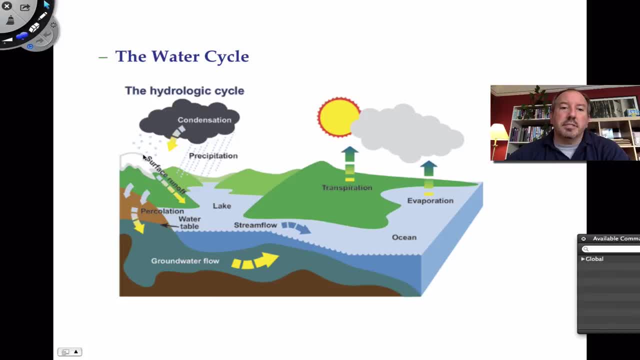 called lakes, and so if it's up at a higher altitude it could even snow, and so you get some snow up here, and then, when the snow melts, you have runoff through streams. Now some of that water on the land can actually penetrate the soil sort of. I like to think about that as sort of like a coffee. 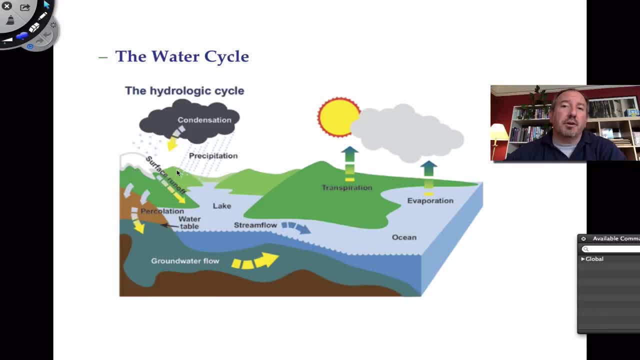 maker. when it's when the water's raining down and it's going through the coffee grounds, it's called percolation, and so this is the source of groundwater as well, and so all that water- fresh water- can run down streams and rivers and then ultimately transport itself back into the. 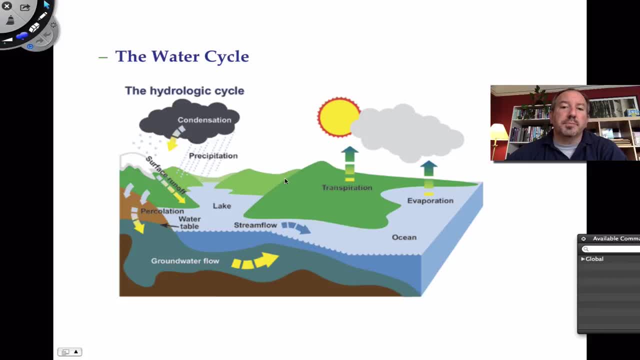 ocean. and so this little notion over here- transpiration, let me animate it to make it a little bit larger. you might be familiar with this, the fact that, for example, I'll just draw one leaf- when water travels into the roots of a plant, it's pulled up through the 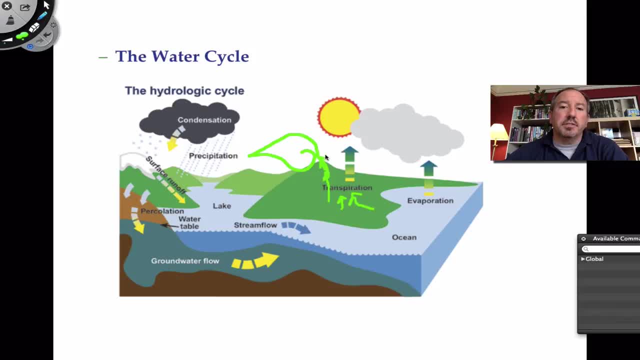 ideas of cohesion and adhesion, and so this is a negative pressure which causes the water to move up a plant and then ultimately evaporate from the leaf. and this is what causes water to be able to move up a tree. it's called transpiration, and so 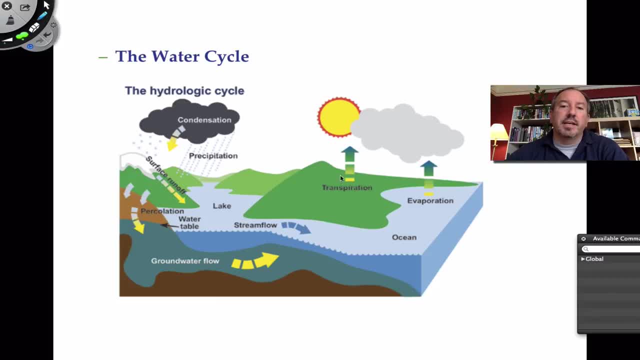 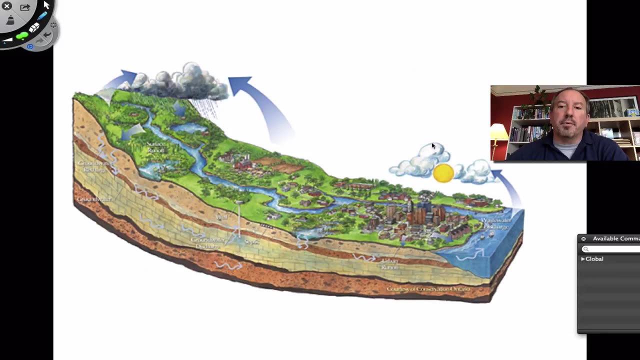 basically, it's the evaporation of water through plants, and the reason I bring that up it's fairly significant. so the water is is being transpired, and that's part of the hydrologic cycle as well, or water cycle, and so here's another diagram of this, and so here's the water evaporating. 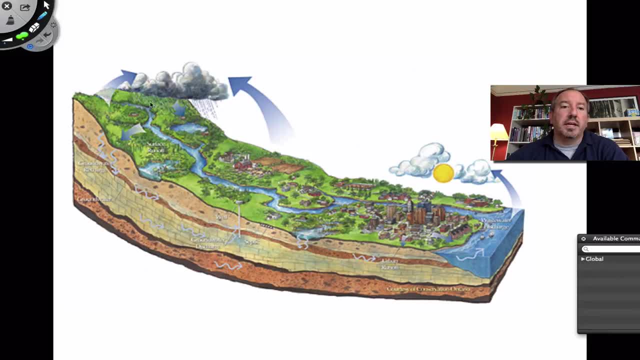 and condensing into clouds, and then here it is precipitating, and so the water can travel in a river again. rivers are one directional. it could actually percolate into the water and be stored in the form of groundwater, or it could be trapped in lakes and as the as the rivers meander down. 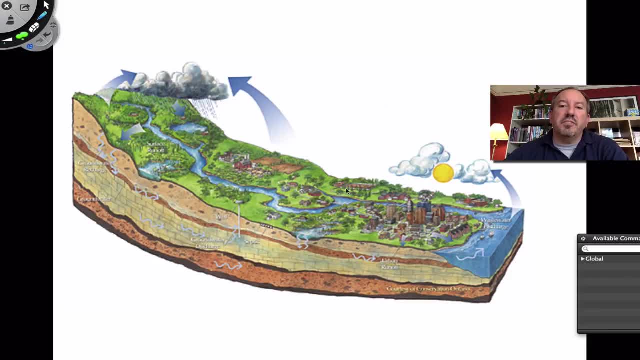 usually the slopes in one direction. it can even fan out into regions called the delta, where the water is meeting the ocean, and sometimes you could even have a mixture of fresh water and ocean water, which we like to call an estuary. okay, so the water cycle is kind of a physical 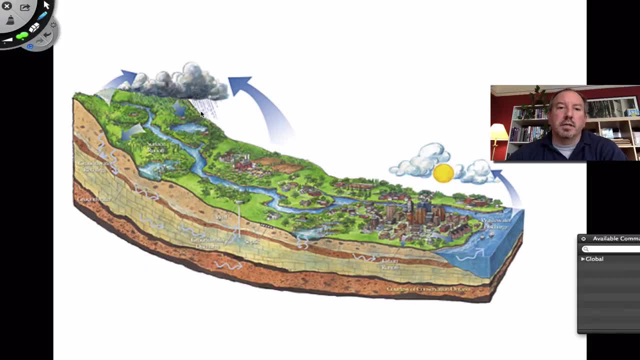 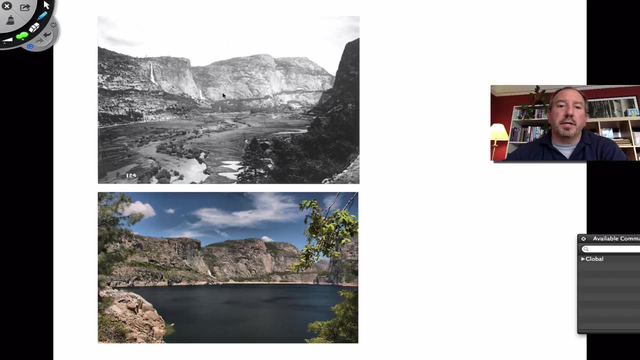 phenomenon has to do with evaporation and condensation, precipitation, and it's quite important to us because, again, all life it requires water, and so I just wanted to point out an area I was mentioning, Waupama Falls in Yosemite, which is right here. this is the great. 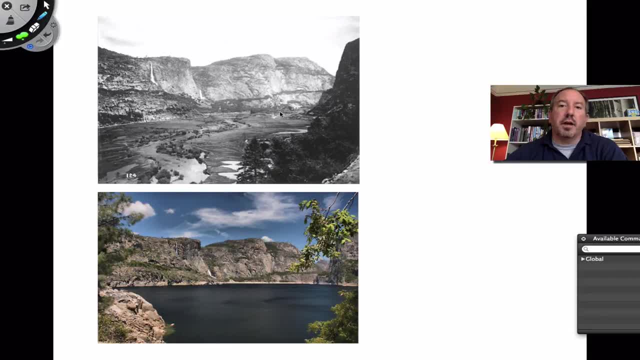 river in California that bisects Yosemite National Park. it's called the Tuolumne River, and this is the Hetch Hetchy Valley. and what's interesting is this Hetch Hetchy Valley no longer looks like this. Hetch Hetchy means grassy valley, and this is the Hetch Hetchy Valley. and this is the Hetch Hetchy Valley. 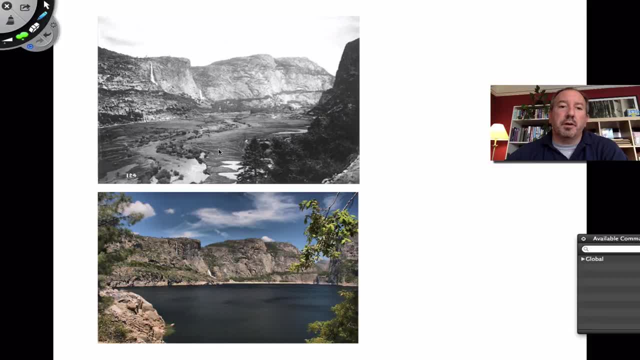 grassy and it was once thought by John Muir to be one of almost as beautiful or as beautiful as the great Yosemite Valley, but unfortunately it was decided that a dam needed to be put right here and block the Tuolumne River and it's called O'Shaughnessy Dam and you can see below that. 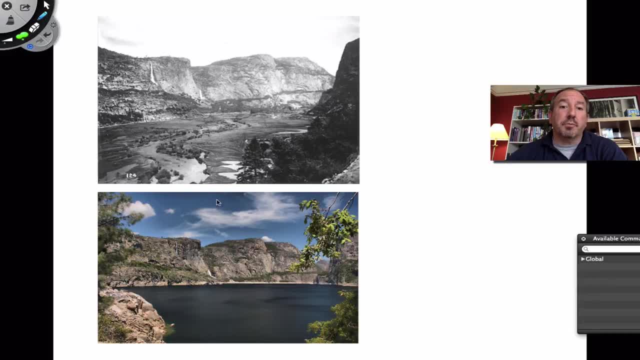 the dam was built- it was finished in around 1923, I believe, and what you see is this big body of water, and we use this water now in the bay area for drinking water, and so it's rather critical, and so maybe someday though, we will eliminate the dam and we'll let the valley 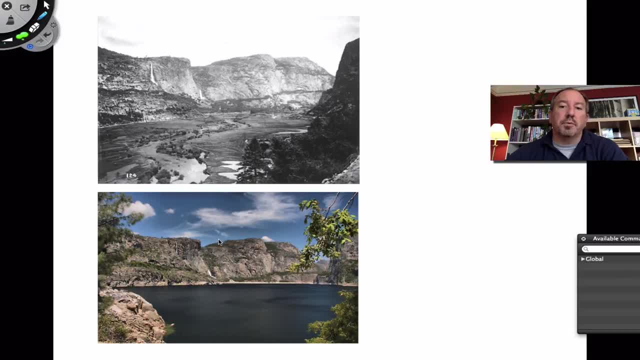 restore itself back to its normal condition and it's like: well, what are we going to do with the water? perhaps someday in the future we'll be able to be able to drink the marine water and be able to remove the salt from that water inexpensively, so that it's more economically feasible. so that's. 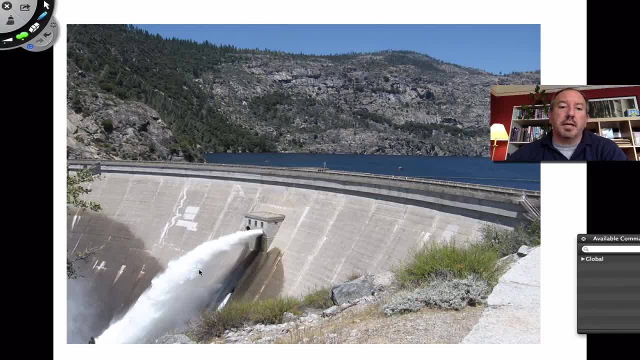 our hope for the future. here's a picture of us O'Shaughnessy Dam and this is the fresh water that's located here in Hetch Hetchy in Yosemite, which is the main drinking water for San Francisco, as I mentioned, and also the city uses a lot of this water pressure for hydroelectric power, which 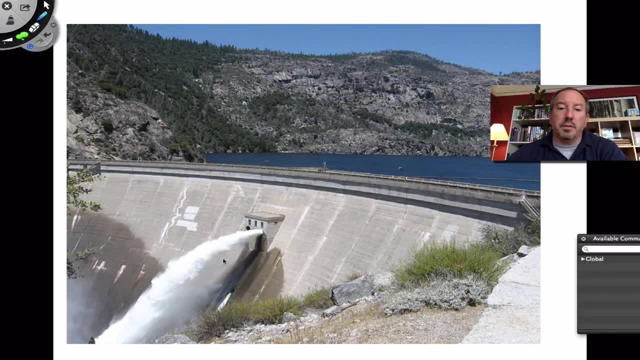 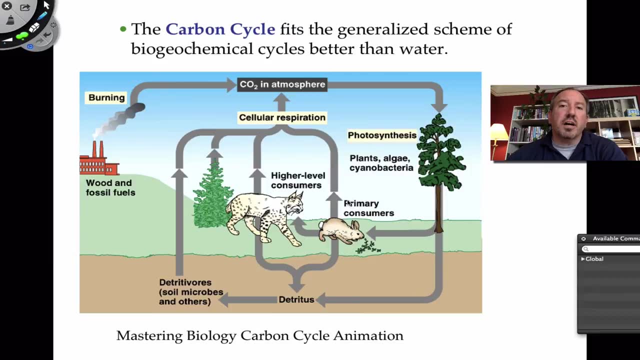 is a great source of energy, which is not a lot of pollution is created, so that's another pro point of the dam. so let's talk about the very first great example of the bio geochemical cycle, and that is of carbon. now, the element carbon cycles like all elements. it's. there's a finite amount of it on the planet. 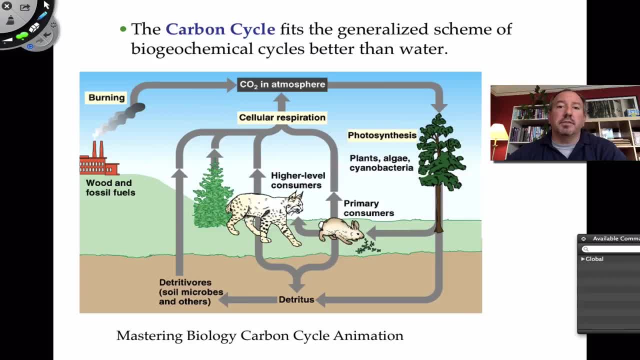 of the earth and basically it's in the air and it's in living organisms, and it's in the soil and it's in the water, and it basically cycles around and around. and so if you're going to discuss a cycle, you know where do you start, and so I could start, for example, in the air, and so 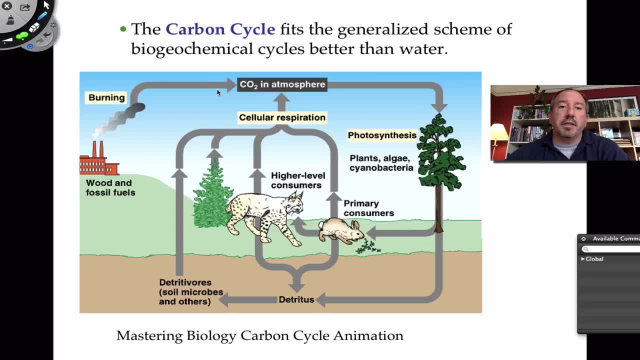 carbon dioxide is a gas and it's found in the air. co2 it's not the only carbon containing gas. there's other gases that have carbon, like, for example, methane gas, CH4, and there's carbon monoxide, CO. but let's talk about co2. co2 is taken in by plants on the land. it's also taken in by algae in the. 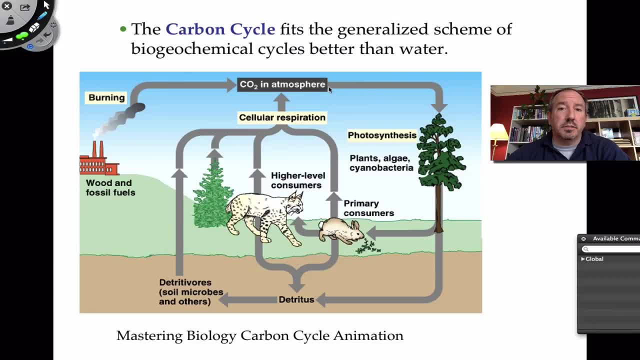 water. it's also taken in by phytoplankton in the ocean, and so when it's taken in, through the process, the biotic process of Analyzing mouth Patternance Photosynthesis, is translated into carbohydrates. and look what's happening. according to what I developed, the process, the biotic process of photosynthesis- it's converted into carbohydrates between egg imbalance- WiederholzJesus- you've heard this phrase before. so C, H, E, Y N, D, E, a little bit over 2,000,000,000,000 times Transylvanian yesterday, he has inherited the Z Robert Schar Company out of on these two rhyme: Analyzing Lawrence offering these commands again. 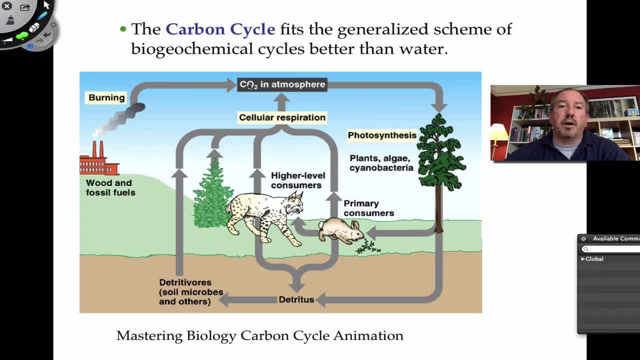 So let me start to illustrate some of this so it's a little bit easier to follow. So that carbon dioxide is then stored in the form of a carbohydrate in either the leaf material or in the trunk of a tree, And so it's stored there. 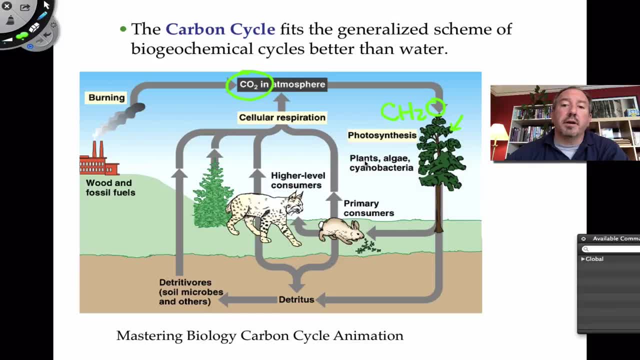 So it's a little bit of a reservoir, And so you can see in the diagram. so it's plant or algae, or even cyanobacteria, which is a word- blue-green bacteria. they can also photosynthesize, So carbohydrates are produced as a result of photosynthesis. 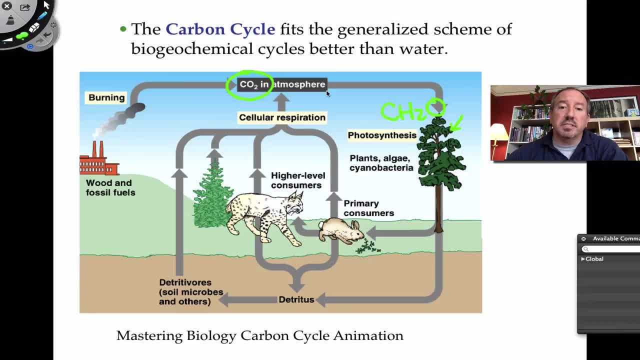 So there's the carbon. Now, tangent to the cycle is the fact that that's not going to happen. unless I don't want you to be confused, but I'm going to bring it up anyway, photosynthesis isn't going to happen without the input of water. 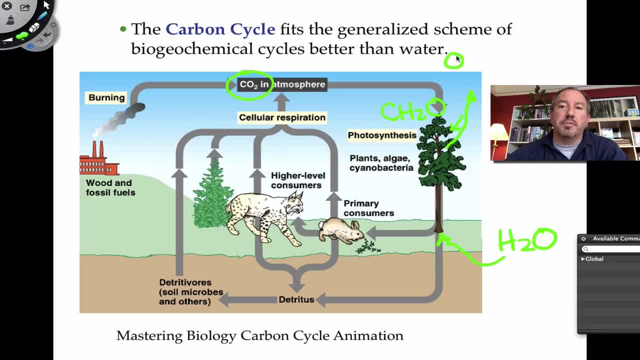 And also as a byproduct. you might be familiar with the fact that oxygen is also produced in photosynthesis, in primary production, But I want to hang out with the Carbohydrate, Because it's the carbohydrate that is then being picked up by the primary consumer. 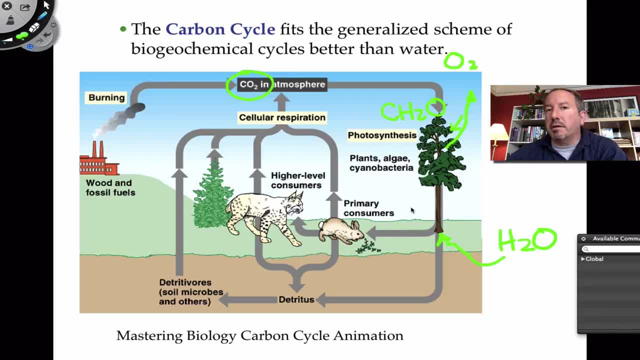 So in this case it's a bunny, but it could be us if we're eating a carrot, or if we're eating some lettuce, or if we're eating a peach or some cherries. Any sort of herbivore is taking in the carbohydrate. 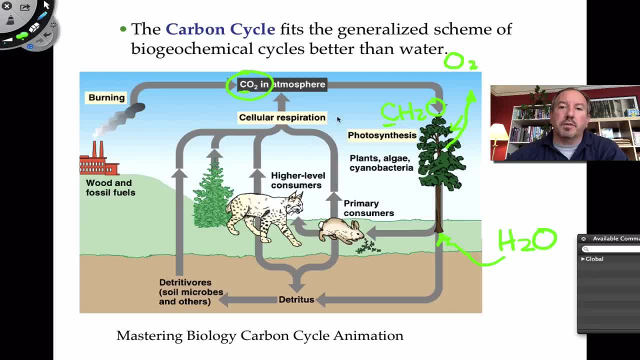 And so that carbohydrate, or that carbon- this is what we're focusing on- the carbon- is going into the herbivore And it's being burned. When I say burned, I mean respiration, So cell respiration, So oxygen is reacting with the sugar. 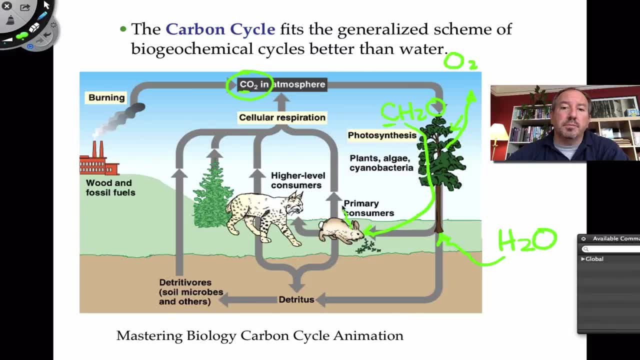 And, as a consequence, of respiration- hope this isn't too confusing. So respiration, it's the burning of sugar with oxygen is then going to release carbon dioxide back in the atmosphere. It's the gas that we're breathing out, So that's carbon dioxide. 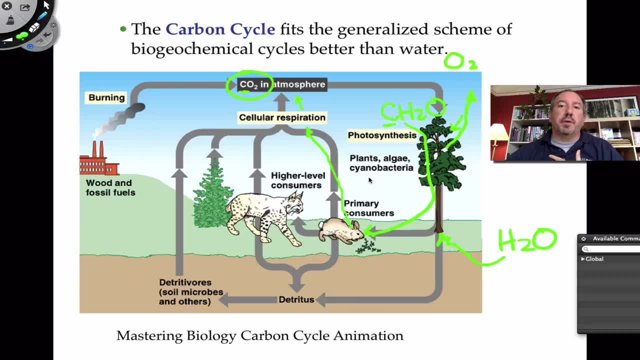 So I'm burning the sugar. I'm burning the sugars that are inside of me that I ate earlier in the day, So that's cell respiration. Now, hopefully, I don't take myself out of this equation, because this is part of the trophic level. 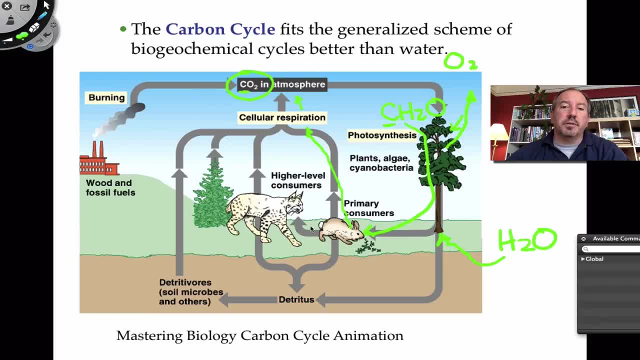 So a nice little bunny might get eaten by a higher level consumer. So in other words, this cat's going to come along and consume it. So the organic- when I say organic compounds now it could mean sugar. In other words, the bunny does have sugar in it. 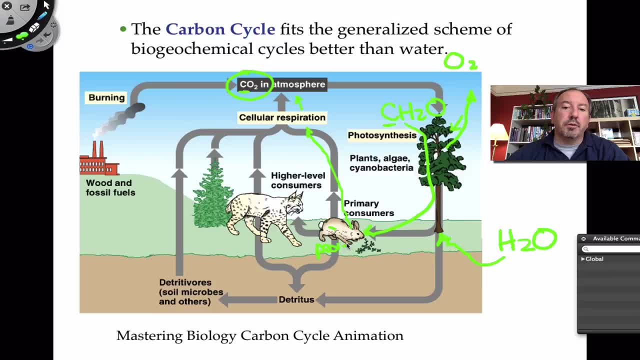 It could also mean organic compounds in the form of proteins or fats like lipids or sugars. So these are all carbon containing and it's like: well, where did the bunny get all these things? Again, it makes some of them on its own, but it gets the carbon from eating the plant material. 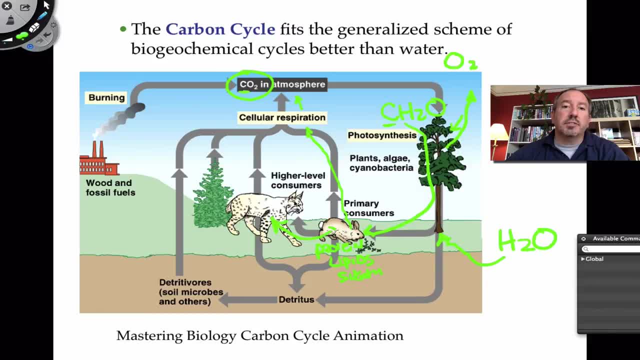 And then that gets moved on to the next trophic level. So if you're a carnivore, you're getting your carbon from eating A rabbit, And now that is also burning the sugar in form of cell respiration, which is putting 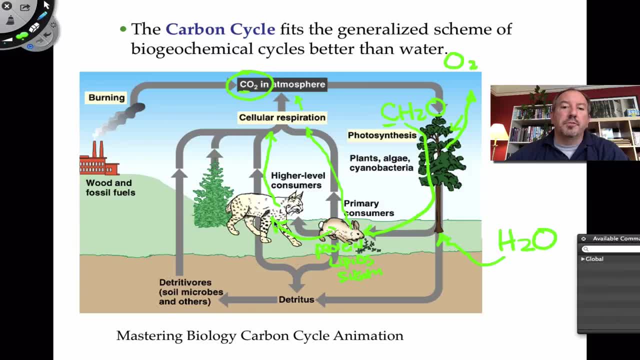 carbon dioxide back into the atmosphere. Okay, So watch this. So let's say that. okay, how come we're including a plant here? Because sometimes it's often forgotten that plants also respire. The reason that they produce the sugar and oxygen is so that they can use it themselves. 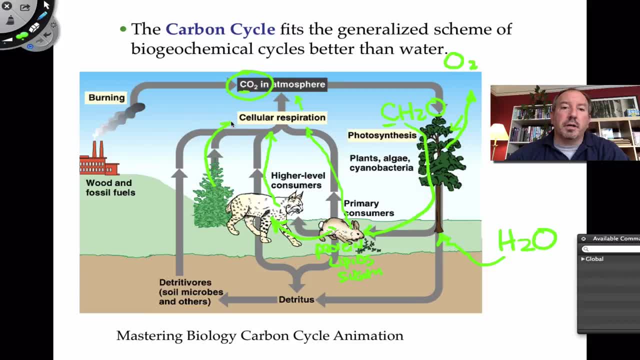 for energy. So plants are also putting off carbon dioxide, So everybody's putting off carbon dioxide, And so watch this. Sorry for being so morbid about this. So when the tree dies and the cat dies and the mouse dies, the rabbit dies everything. 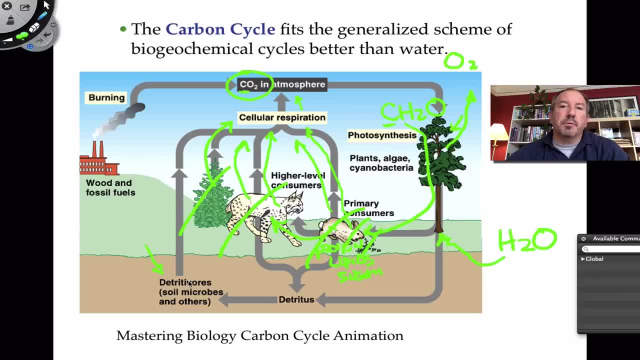 dies, You get detrivores, which are organisms that are eating dead organic material. Now let's look at the decomposers of this, which are the bacteria and fungi. Okay, They're going to be breaking down those organisms, the detritus, breaking down the dead material. 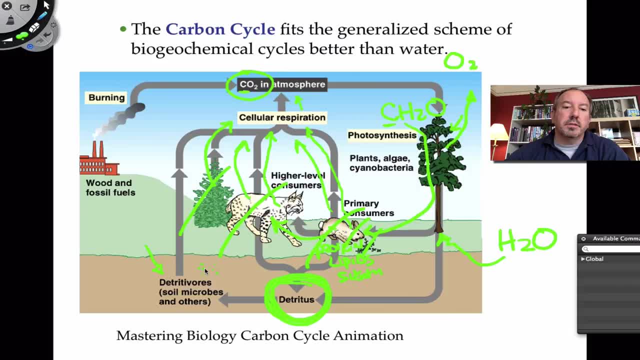 and breaking it down into simple elements. simple elements, And it's the bacteria are going to be consuming those organic molecules for energy And they're also breathing out carbon dioxide, So the microorganisms. so how about this Carbon dioxide's rising out of the soil because bacteria are producing that. 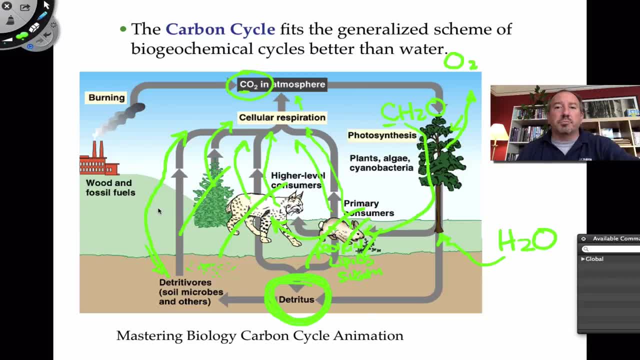 Plants are producing carbon dioxide. We're producing carbon dioxide. Cows are producing carbon dioxide. And so how do you like this? Many, many, many millions of years ago, when the earth was covered by huge amounts of coniferous forest, those trees that passed away, 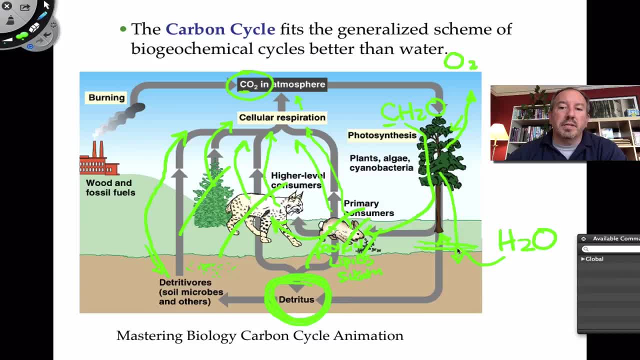 Here's a physical process, or we're built up by pressure and push down and sediments building up all down here like this, And then ultimately what we get in the bottom of down in here we have something called coal and we have oil. Now that was a poor description of the formation of coal and oil. 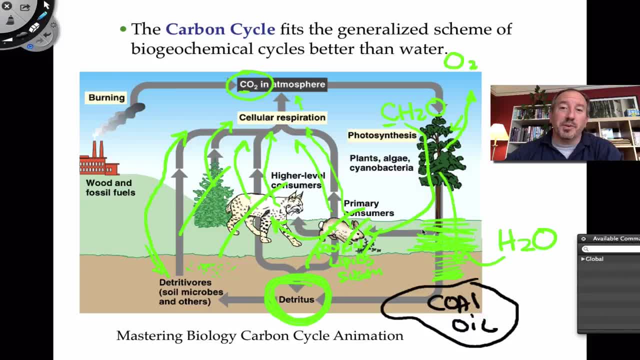 Sorry about that, but take take me on faith on this. If you want to look it up, it's fine. at the forests are broken down into coal And oil, which are these massive reservoirs of carbon molecules. So these are hydrocarbons, lots of carbon here. 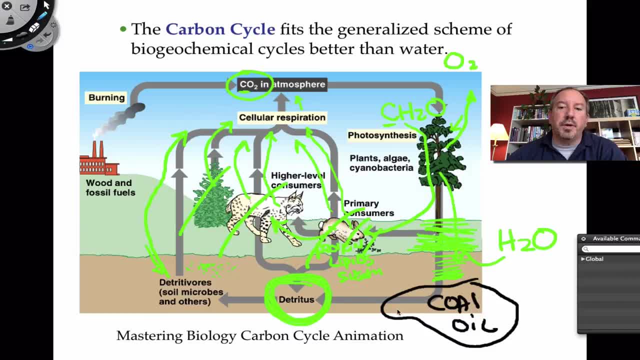 Where did the carbon come from? photosynthesis. And so what we have done, humanity, let's put us over here. We take these carbon compounds, the oil and the coal and even wood, and we burn it again. Same, It's the same reaction as cell respiration. 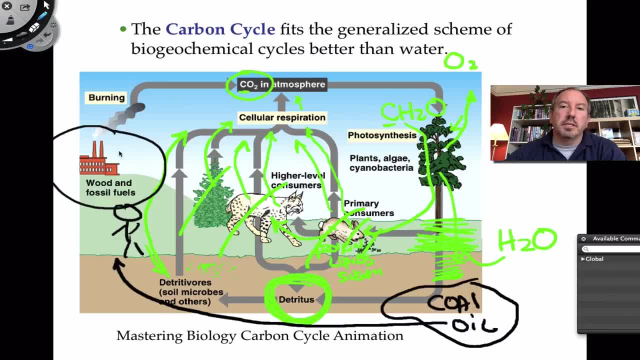 We're burning these in factories, Yeah, To produce heat and energy, and we can power our cars and warm our homes. You know this. but as a result, carbon dioxide is produced and you're like, wow, there's a lot of carbon dioxide being produced. 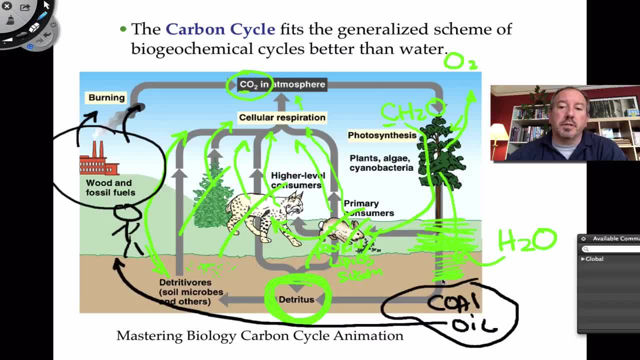 Yeah, Because combustion reactions, in other words burning fuels, produces carbon dioxide. But then you know, all things being said, you might get worried, but actually the level of carbon dioxide is really just a little under 1% Of what air is carbon dioxide. 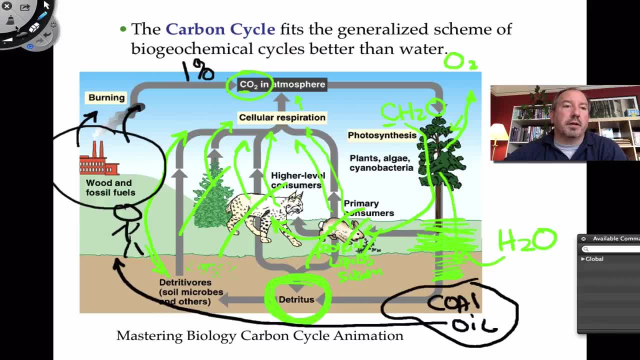 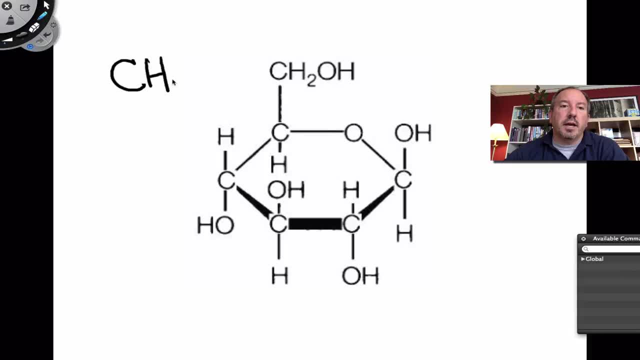 So here's a brief look at the carbon cycle. Hopefully that wasn't too busy. Now, when I was mentioning carbohydrate, I was saying: you know, see, uh, H2O carbohydrate. but here's a picture of what glucose- this is a simple sugar monosaccharide. what it 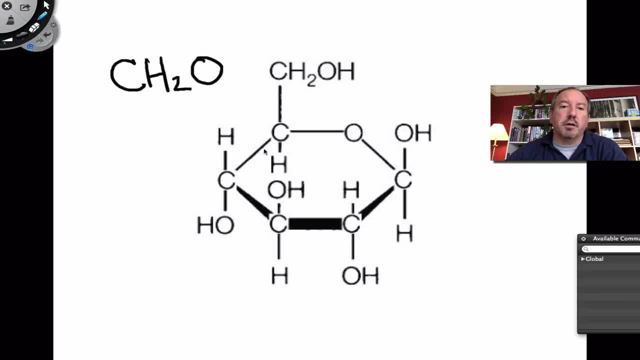 looks like: Here's a carbon, There's a carbon, There's a carbon, carbon and carbon and carbon. If you count them up: 1, 2, 3, 4,, 5, 6.. So if there's six carbons, you see this, you can predict how many. twice as many. 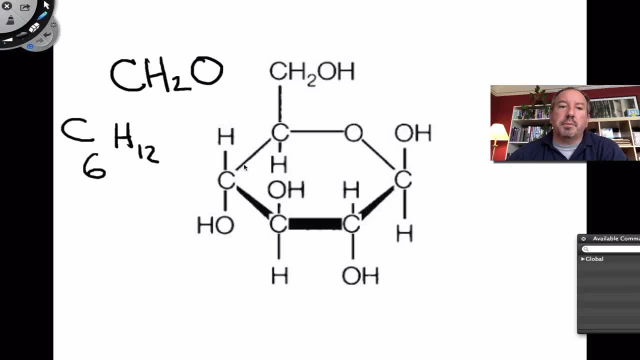 So you'd be like ah, 12.. And then how many oxygens? bup, bup, bup, bup, bup. I don't even have to count them. There's six. See how it's the ratio of one to two to one. one to two to one. 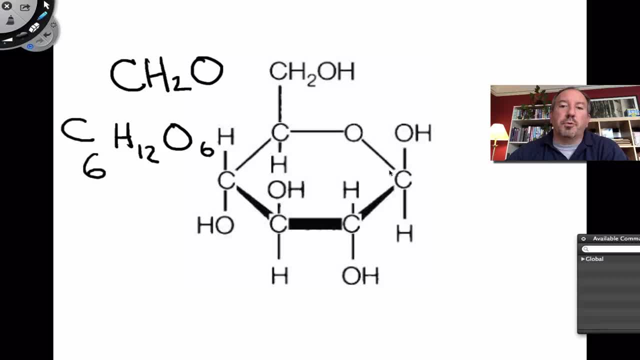 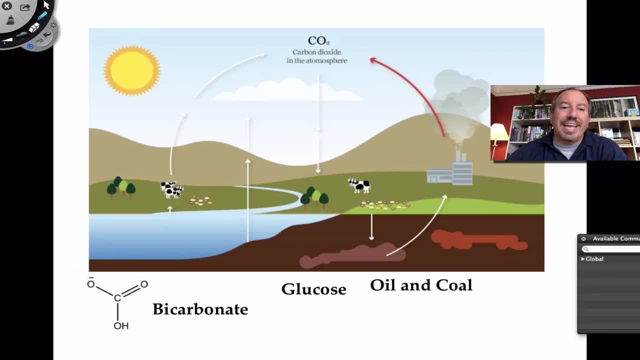 So this is what we're talking about in terms of carbon dioxide is stored in the form of sugar. I thought you might appreciate that. And so factories are producing carbon dioxide. Animals are producing carbon dioxide. How about this? Here's a little trivia. 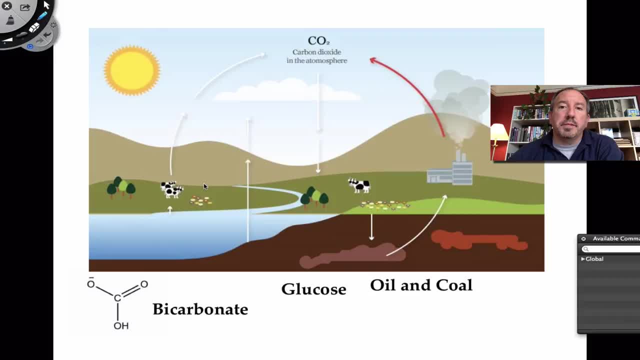 What organisms, what animals are producing the most carbon dioxide? You know like, Hmm, you might say, well, it could be the largest animals, or, but then you'd have to consider which are the most numerous animals. Notice, I mentioned animals because if I said what organism is producing the most carbon, 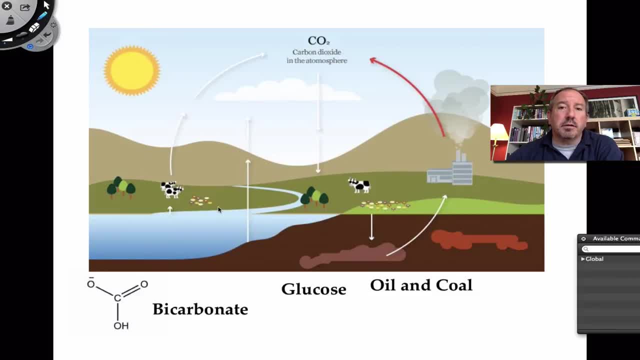 dioxide. you would easily answer that and say that bacteria are producing the most carbon. Yeah, Yeah, Yeah, All kinds of bacteria are producing the most carbon dioxide. But if I say what animal, say what. what's the most numerous animal that's doing this? 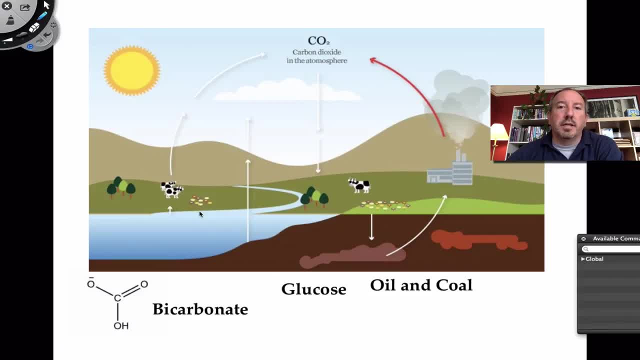 That's eaten a lot of wood and producing a lot of carbon dioxide. that would be termites. So termites make a tremendous amount of carbon dioxide, And actually so do cows as well, And horses and stuff. So what happens is here's the oil in the coal that can be burned into carbon dioxide. 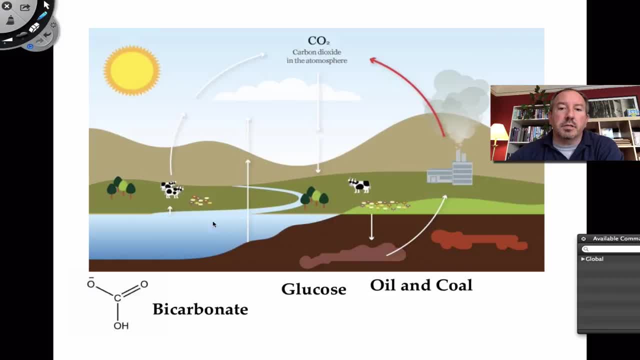 Remember, photosynthesis is what's making the sugar, In other words, glucose. right here, carbon dioxide is making glucose. And then how about this? that carbon dioxide goes into the water, and there's also great levels of primary productivity in the water as well. 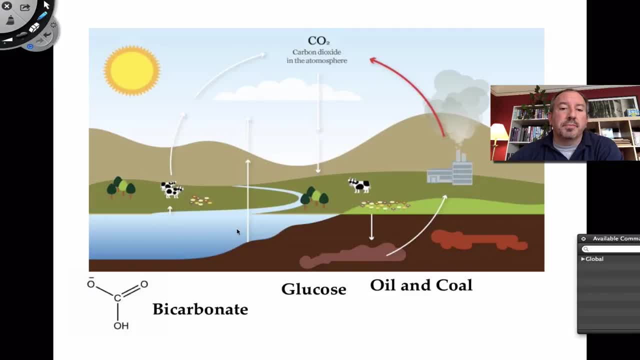 Algae are producing glucose, And that's important because all the consumers in the water need that primary productivity in order to survive. They're the ones eating, And so the carbon cycles happen in the water as well. Now, what's interesting is about this little tangent is that carbon dioxide when it dissolves? 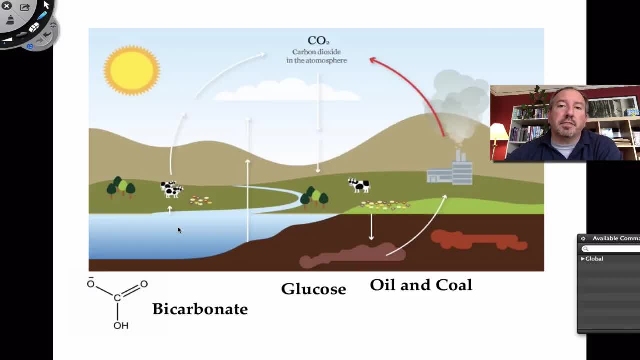 into water, as it turns out. you might be familiar with the fact that carbon dioxide really dissolves easily into water, And that's what we like. carbon dioxide in our water, It's what makes soda, And then we can add some sugar to that and it's carbonated water. 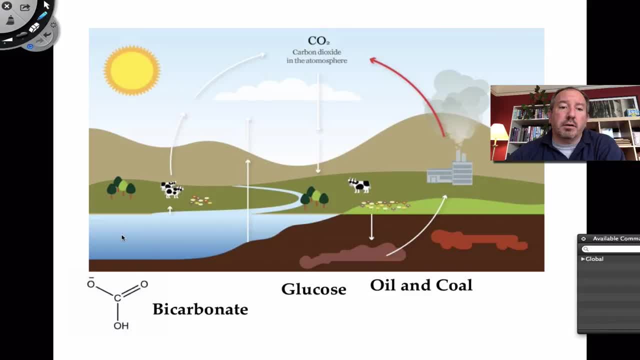 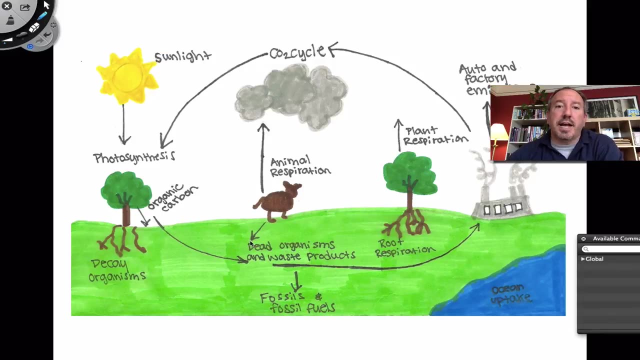 And so when carbon dioxide reacts with water, it forms this product called bicarbonate, And this is actually how a lot of it is stored in water, in this particular structure, bicarbonate ion. And so just a little something there And again, just to final tie it up on the carbon cycle, is that some of the things? is that plants? 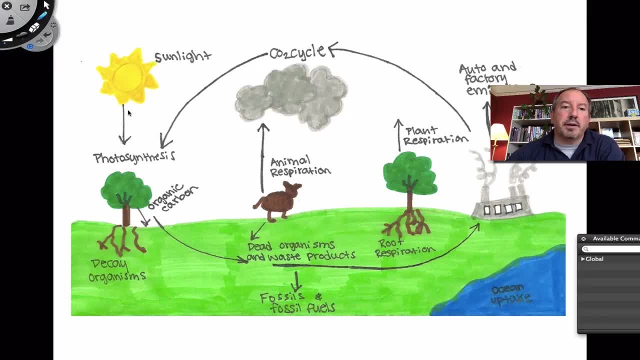 respire, producing carbon dioxide. animals respire and then plants take this up And again factories produce carbon dioxide as well. A concern is that sometimes, when there's lots of fires going, In addition to just the burning of carbon containing molecules, when there's a lot of fire going on, 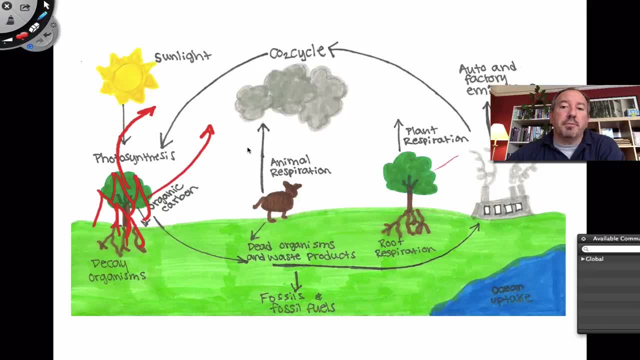 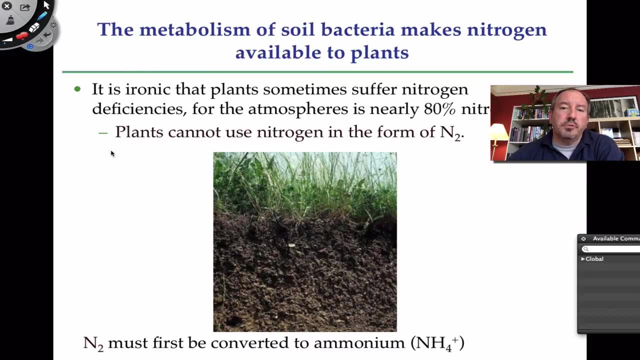 that also increases the carbon dioxide in the atmosphere, So we have to be careful about that as well. Just want to point that out. So now let's draw our attention to the nitrogen cycle. Now the nitrogen cycle is so very important, And let me explain why that is the case. 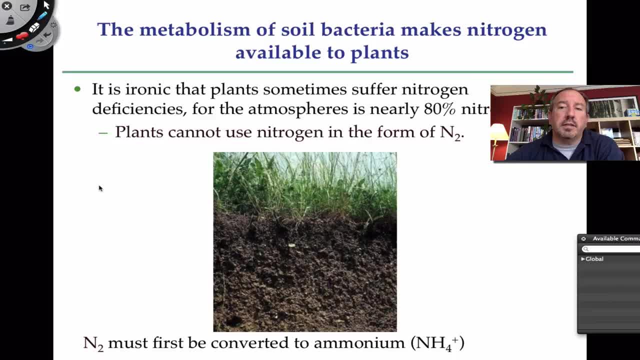 Because nitrogen. you may not be able to appreciate If you're just beginning studying biology, but I'll just say this: that nitrogen is found in very, very important molecules such as protein, And so proteins- in order to make a protein, you need nitrogen. 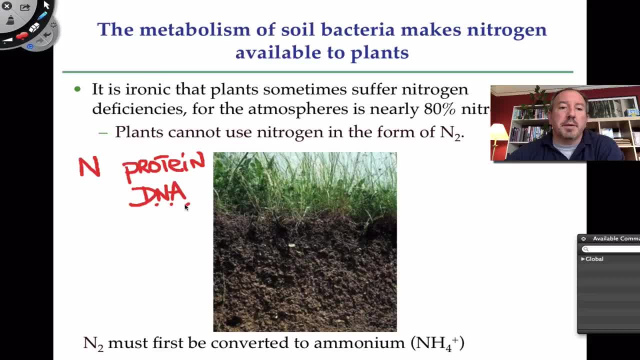 And then let me throw this out. You might have heard of this deoxyribonucleic acid and ribonucleic acid. These are important compounds, biological molecules that need nitrogen in order to be produced, And so I can ask you this: 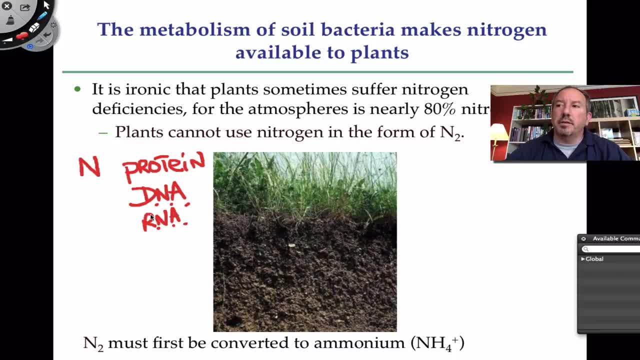 So where do we get our nitrogen? And like, well, again, we get our carbon from eating both animals and plants and we get our nitrogen from both eating plants and animals. So we get it from eating, but ultimately it comes down to plants. 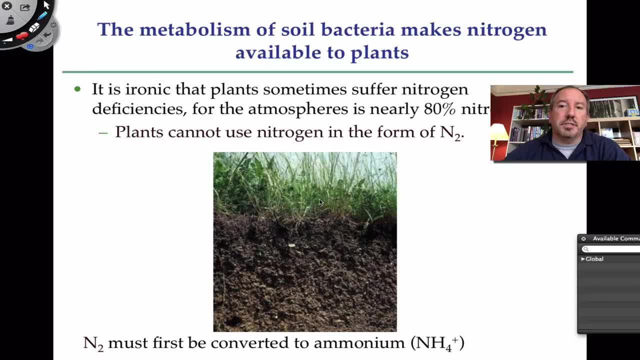 It comes down to where are plants getting nitrogen, And so this is why the picture of the, of this grass here in the soil- Because it talks the metabolism of, in other words, the chemical reactions of bacteria and plants- are really going to be what makes 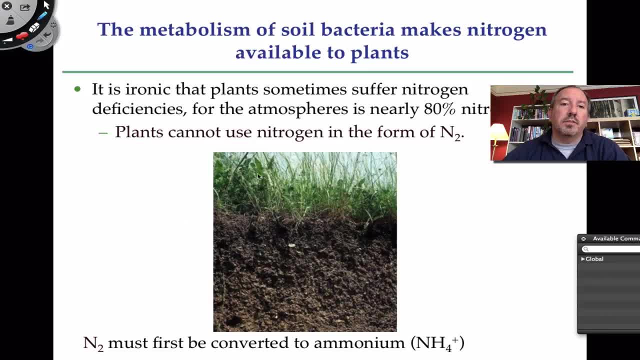 nitrogen available to us if you want to make it human centric. And so what's ironic? the beginning of the nitrogen cycle discussion. what's ironic is that in the atmosphere- remember I was saying that that carbon dioxide is less than 1%- 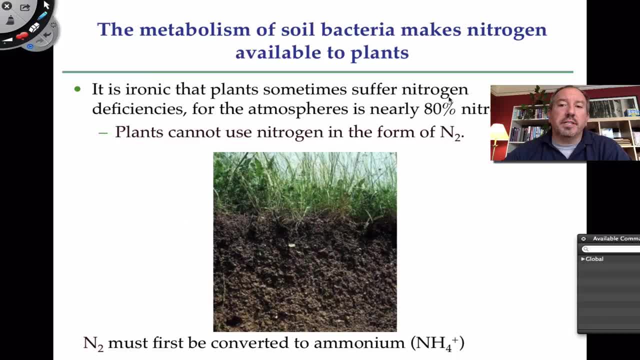 You ready for this Atmospheric uh? nitrogen is 80%. Okay, So in other words, out of a container of air, if you get a simple container of air, 80% of air is nitrogen gas and nitrogen gas is a. the molecular formula is N2.. 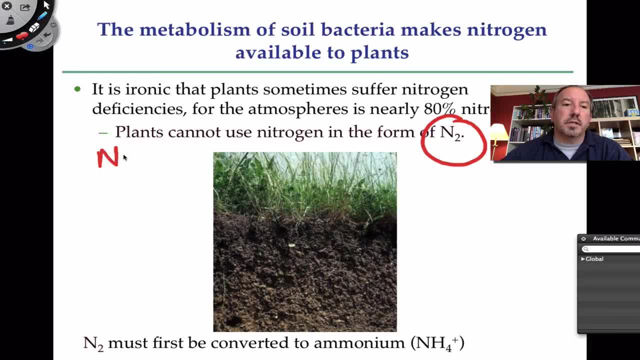 Let me sort of do that. It's N2, which looks like this triple covalent bond. So 80% of air is nitrogen gas, And so you might be thinking, wow, all plants have to do is breathe it in, and they're good. 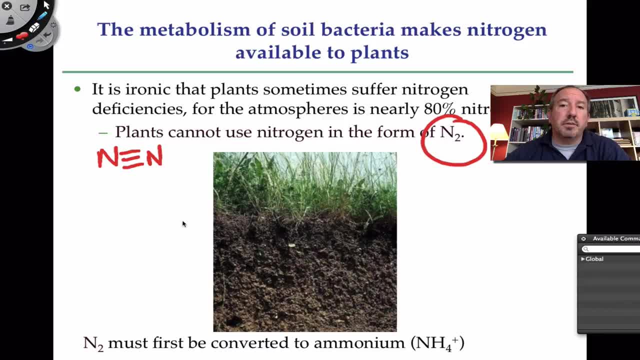 They'll be able to have nitrogen and be able to To produce their proteins. Now, unfortunately, plants cannot assimilate, In other words, transfer nitrogen gas into usable compounds, So they breathe it in, they breathe it out, And so what's going to happen? as it turns out that bacteria are really 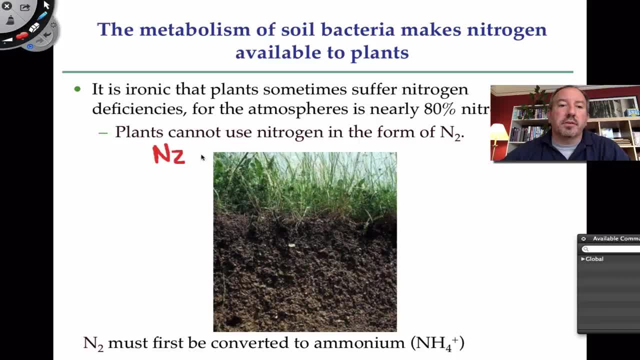 really, really important here. And so the nitrogen gas travels into the soil like this travels into the soil. Now, it's not going to travel into the soil. If you put concrete Concrete here, that's going to be a pen, that's going to be impenetrable, but say it's outside. 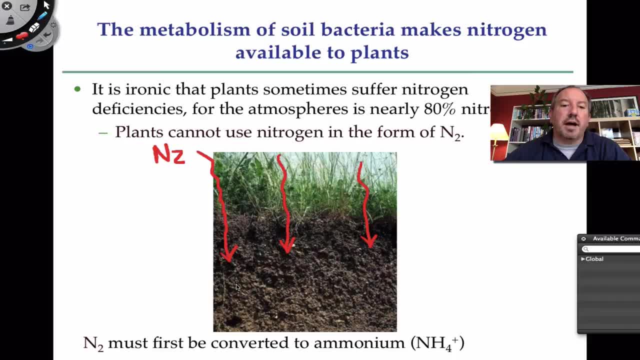 And so the nitrogen gas is going into the soil And, as it turns out, there's lots of different kinds of bacteria And we're about to talk about them. There's all kinds of bacteria. I'll just make it really large so you can see it- but really they're invisible because they're microscopic. but there's bacteria that will take this nitrogen gas and they'll convert it into another chemical called ammonium, which is N. 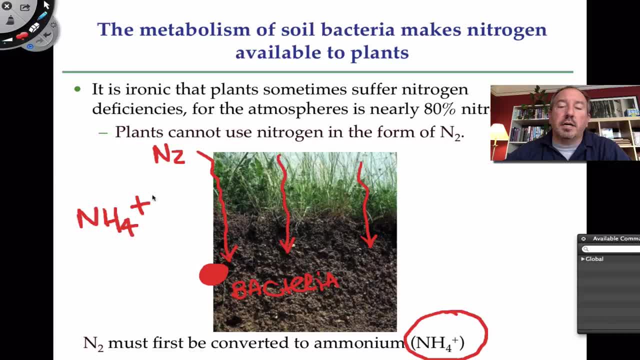 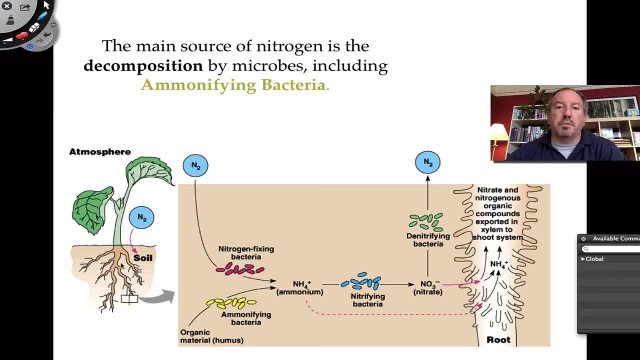 H four plus. and it's an ion because it has an electrical charge, So they're able to take nitrogen gas and turn it into ammonium. You're like, well, why is that important? Well, it's because the ammonium- if you look down in this diagram, the ammonium is something that can diffuse into the roots of the grass and the plant can then take the ammonium. the NH four plus. 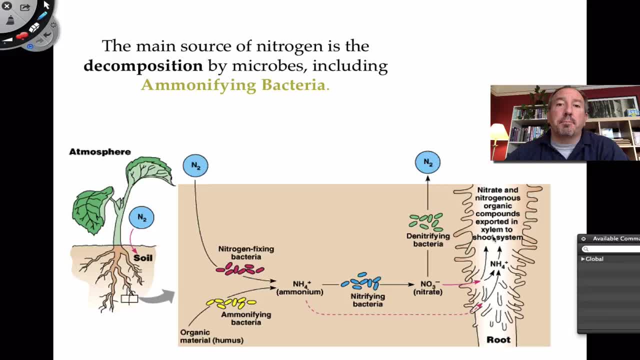 So it's a very good way to break that apart and use the nitrogen to produce protein. First it creates amino acids, which are the building blocks of protein, but ultimately they produce protein, and then we can come along and eat the plant and get the protein. 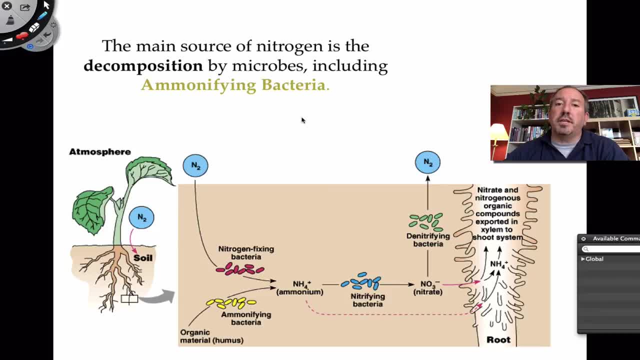 That's how we get protein: from eating plants or eating an animal that has eaten a plant. And so how does the plant make the protein? It First Has to Absorb ammonium in the soil. And who's going to do that? 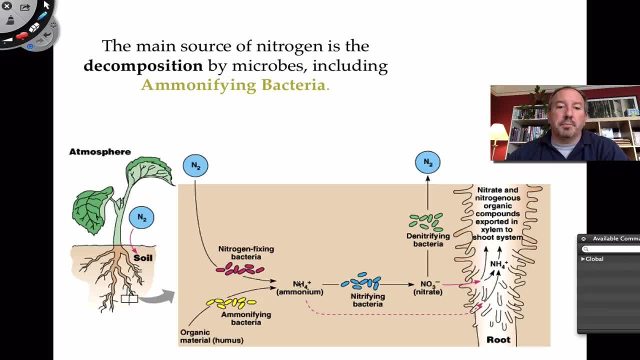 Who's going to produce ammonium? Well, I was mentioning this, that there's a type of bacteria in the soil that's capable of breathing in nitrogen gas. It's called nitrogen fixing bacteria. Now, I know that this might be a little overwhelming to you, because it's like a throne. 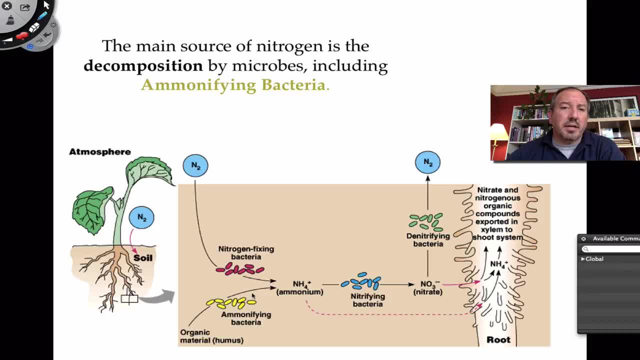 I'm going to come strong with different kinds of bacteria here and I'm going to name- I'm going to name them- three different, four different things, And so it's like, oh you know, but again it's something that is so critical- and I don't want to say that for everything, but this is extremely critical and it's worthwhile for us to pay attention to it. 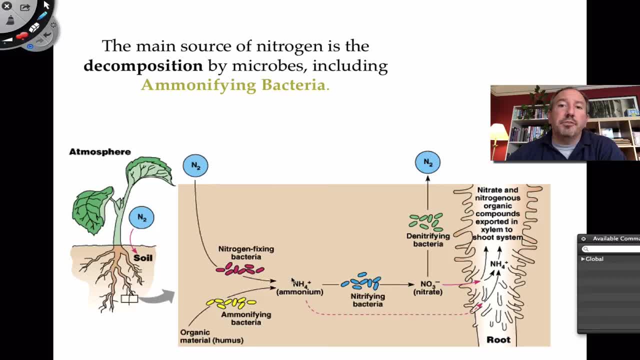 But just like anything, just to pause for a second, if you're just meeting people for the first time and people are introducing themselves to you, they're like: hey, my name's this, my name's this, It's sometimes it's fleeting and you forget their name and that's, and that's kind of common. 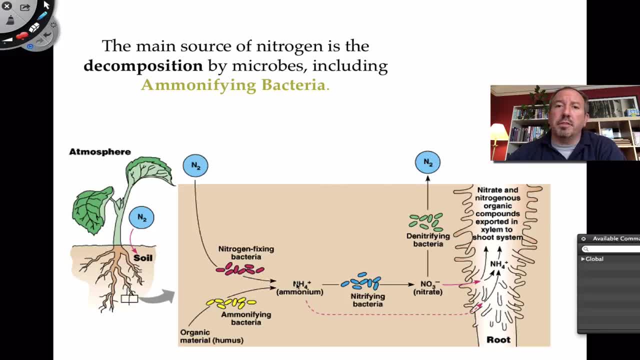 But the more you spend time with them, the more you get to know with them and you start to develop a relationship. the names become really important and you get to know them And it's like almost impossible to think of them other than their name. 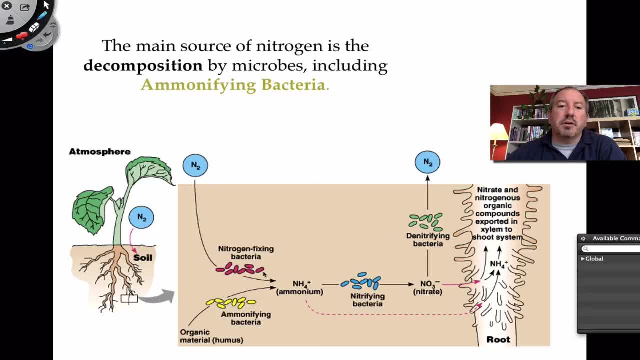 And so I just want to point that out. These are called nitrogen fixing bacteria. They can take nitrogen gas from the air and turn it into ammonium. But I want to first, before I go into nitrogen fixing, I want to talk about another class of bacteria that's in the soil. 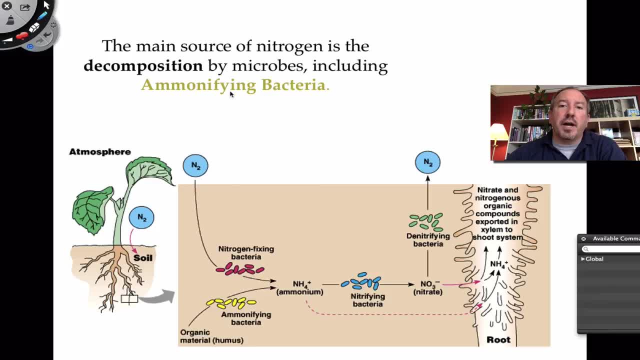 This is underground, This is in the soil Close up. Ammonifying bacteria- Now, ammonifying bacteria are basically bacteria that will take dead organisms, In other words detritus. So a dead plant, orange peels, banana peels, corn husks, a dead rabbit or dead ants or leaves or anything detritus, any organic material, any organic material. 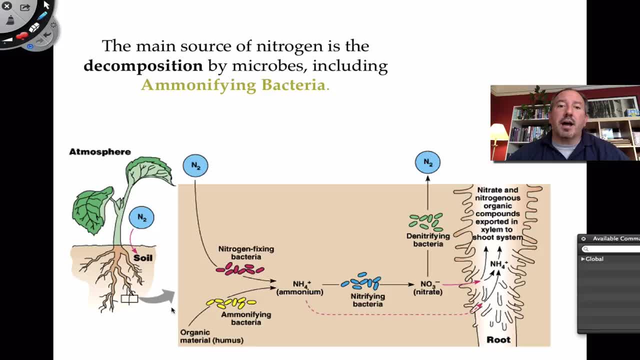 Like, For example, in your compost pile at your house in the backyard, any organic material. you're going to get bacteria called ammonifying bacteria, shown here in yellow. They're not really yellow, but ammonifying bacteria will break down those nitrogen compounds such as amino acids, and they'll break that down into ammonium. 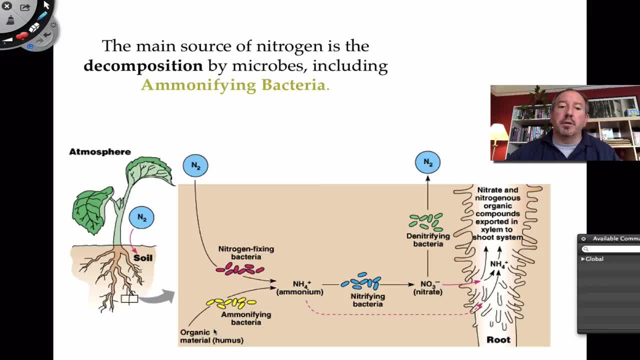 And what that does is it sort of like, if you will, Makes it smaller. That's a simplification. Makes it smaller in your compost pile because you know compost. the goal of compost is to make good soil, So your compost pile after a while is going to have a lot of ammonium in it. 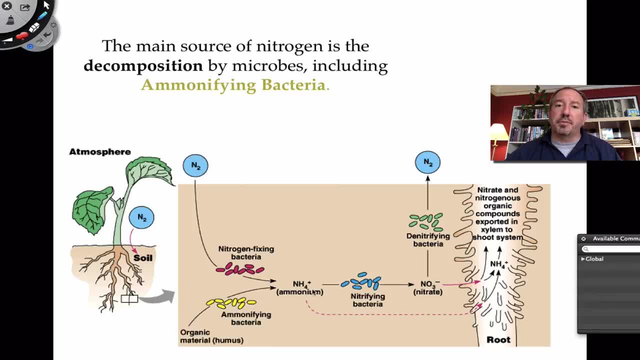 Can you appreciate? that, for once, was like food scraps. It's now ammonium And you're like, gee, the soil's really good. Why is the soil really good? Because it has a lot of ammonium in it. And what is the ammonium going to do? 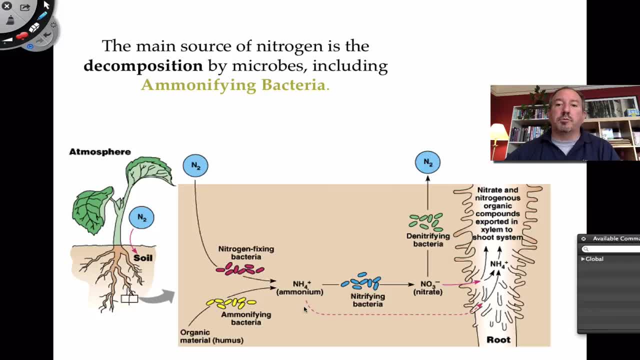 Well, when you take that soil and you put it in your garden, where you're growing roses, for example, or you're growing a vegetable garden like zucchini, that ammonium is then going to be taken in by the plant And it's going to be able to produce its own protein, amino acids, and it's going to thrive. 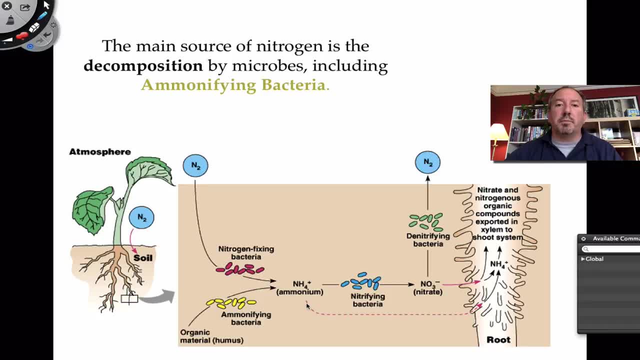 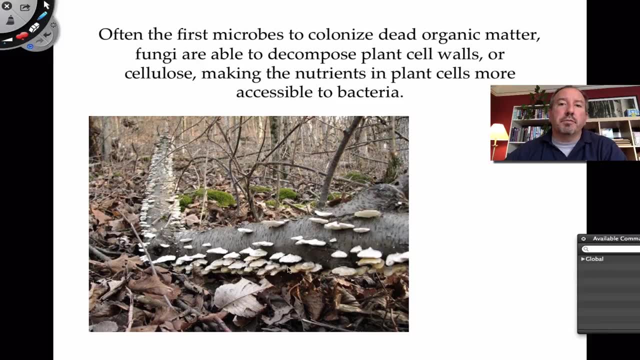 So that's what we mean by good soil. Good soil has ammonium in it, Okay, And so what's interesting is in nature. you know, nature composts on its own. It doesn't need humanity To think that it's helping out. And so when a tree falls, it's going to get broken down. But one of the things is bacteria sometimes, interestingly enough, have a hard time breaking down the proteins or what have you in a tree, because the cell wall is so difficult. 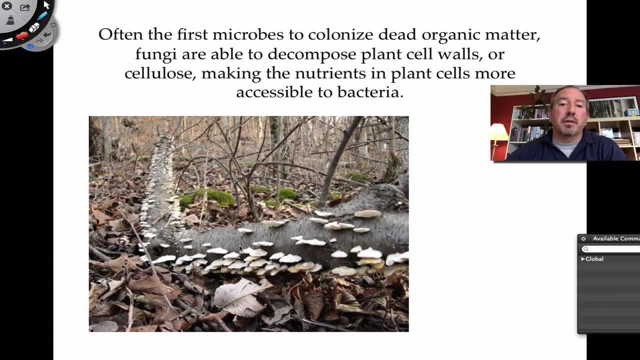 And so oftentimes you need the help of fungi. So there's mushroom and other fungus produce these really interesting enzymes that will break down cell walls, And so fungi break down the cell walls and then that makes it accessible to bacteria, the monofying bacteria that will turn the organic compounds that have nitrogen in it into ammonium. 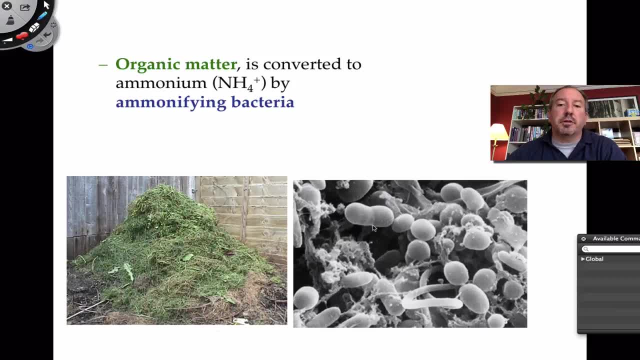 So these ammonifying bacteria, this is an actual picture of them. They sort of look like little cotton balls. They're circular, called cocci cocci bacteria, Kind of a weird name. So here's your compost pile, And so what's happening? 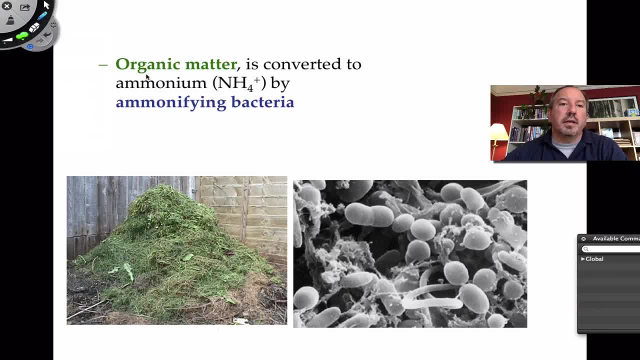 Let me illustrate this. What's happening in your compost pile is that organic material which is like the leaves, so all this leaf material. okay, what's inside of the leaf material? The leaf material has things like amino acids in it, And now if I were to draw a bunch of amino acids, I might make it like this into a chain. 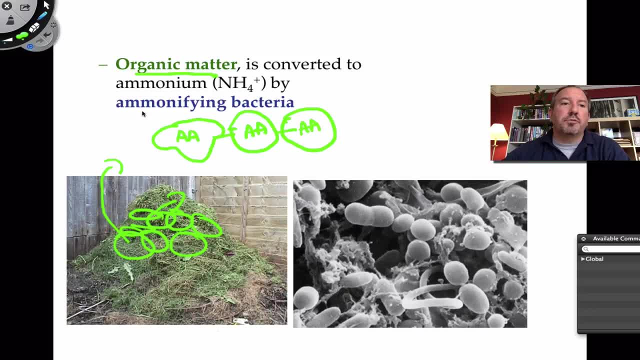 And a chain of amino acids makes a protein. But if I were to draw one simple amino acid, I'm going to draw a chain. I'm going to draw a chain. I'm going to draw a chain. I'm going to do that for you. 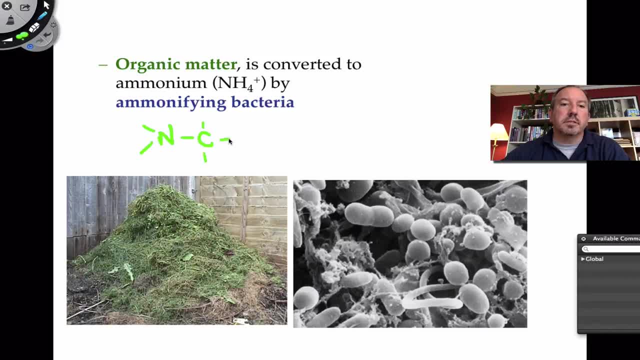 I'm going to say that an amino acid looks a little bit like this: They don't get overwhelmed. So here's an amino acid, Okay, And so this bacteria right there is able to take in the plant, which is the organic material, the plant amino acid, and sort of just rip it apart like this: 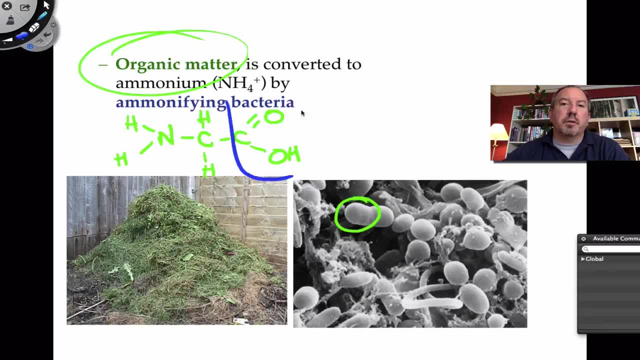 Let me get this. So it rips off this group, this carboxylic acid group, and it rips off the R group, And then it rips this Ammonium off And it turns it in. I'm sorry. 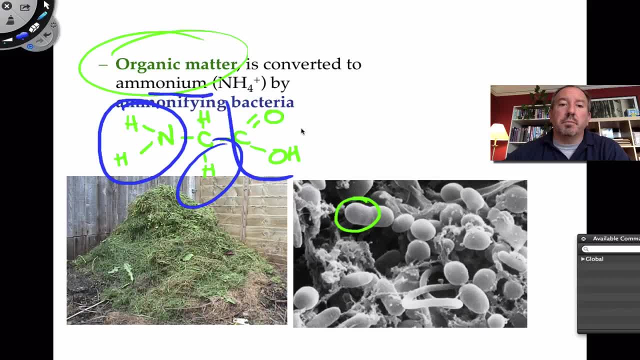 This amino group And it turns it into ammonium, And so what it does is it's producing ammonium right there, And so now that is prevalent in the bottom of the compost pile. This is our goal is to make a lot of this. 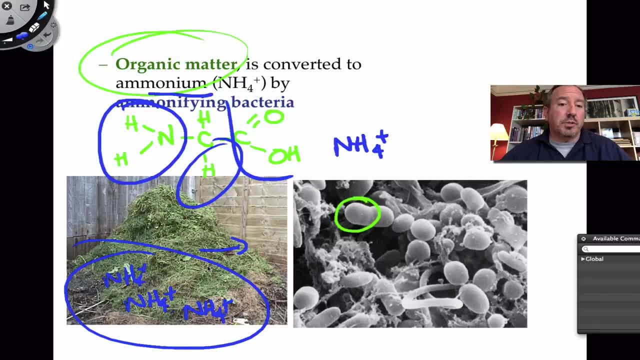 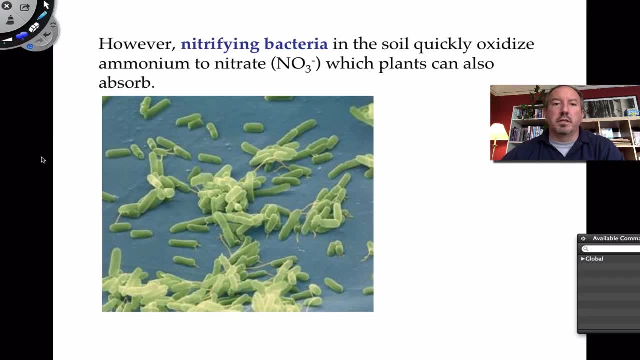 Why do I need a lot of this? Because plants, when you feed that soil to your garden, it's going to appreciate. It's going to appreciate all of that ammonium ion. Okay, Now here's something, And maybe this will be disappointing, but there's another step in this process. 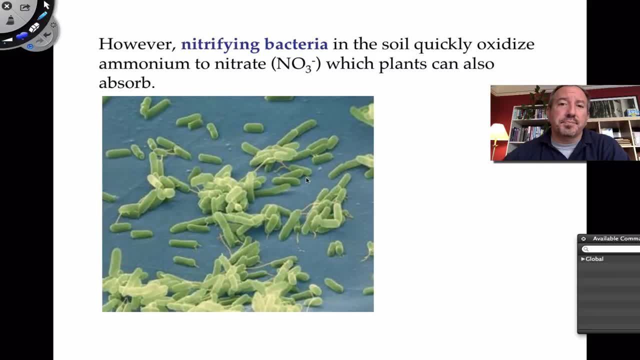 I think it makes it even more interesting. It's all about your attitude. As it turns out, grass in your garden, you know, can take ammonium, But it actually prefers to take nitrogen in the form of nitrate, And so there's another kind of bacteria. 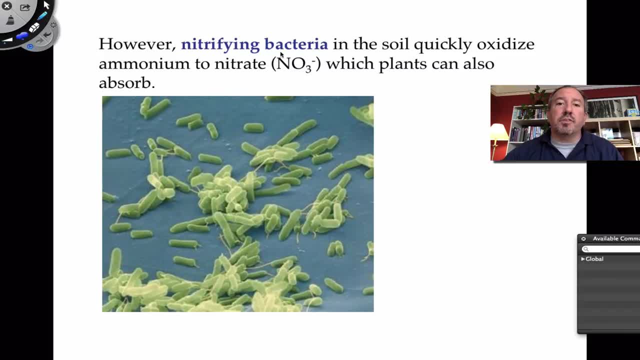 And the soil called nitrifying. The name sort of says what it does. It takes the ammonium ion and it converts it in. Instead of NH4+ it turns it into NO, which is oxygen 3- And plants love that nitrate. 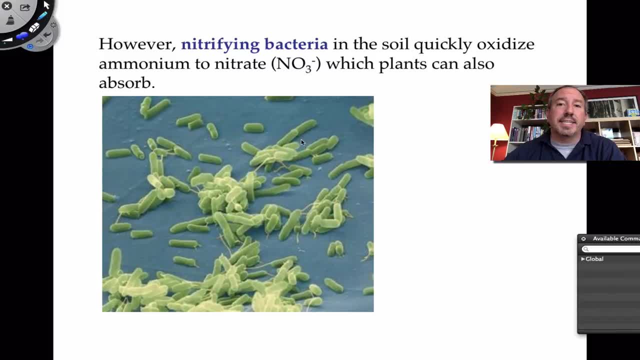 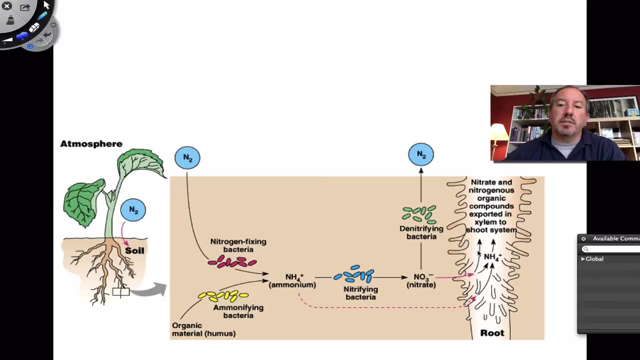 And it can also turn it into NO2, nitrite, And so check this out: Nitrates and nitrites are over here in the soil And plants really take that in Extremely, Extremely well, And who's doing it is the nitrifying bacteria are doing that. 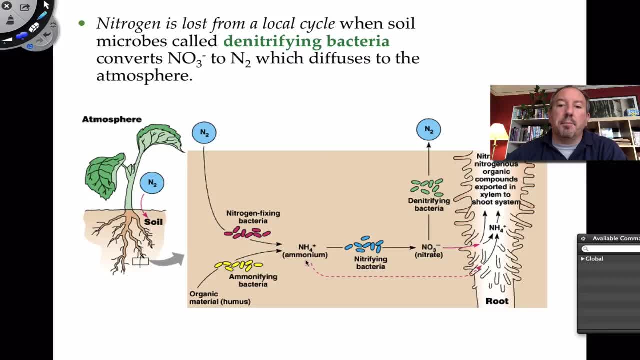 So the nitrifying bacteria can turn ammonium into nitrate and nitrite, And so plants can take that in. So to complete the cycle there's yet even another kind of bacteria called denitrifying. Denitrifying bacteria will take in also in the soil- nitrate. 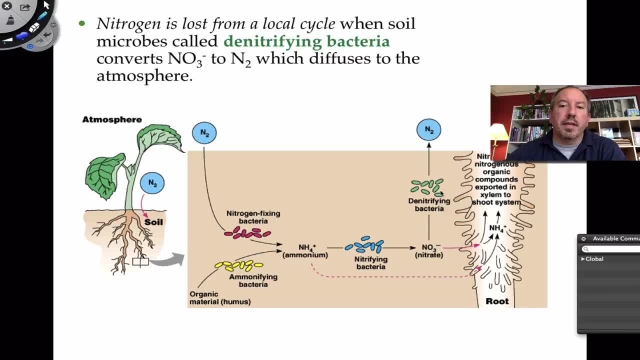 Now it'll take in nitrate and it'll break down the nitrate back into gaseous nitrogen And so that then diffuses out of the soil. Remember when I was talking to you about the carbon cycle? I was saying that the bacteria produce carbon dioxide when they're respiring and the carbon dioxide's coming out of the soil. 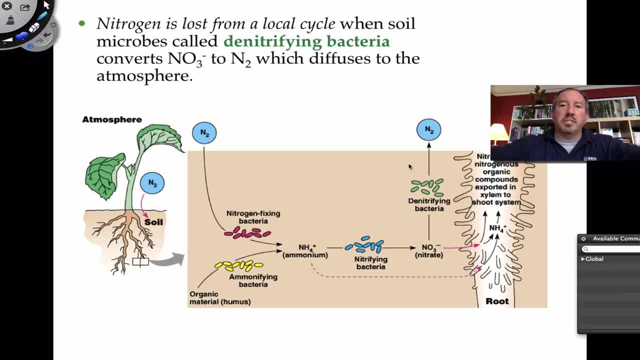 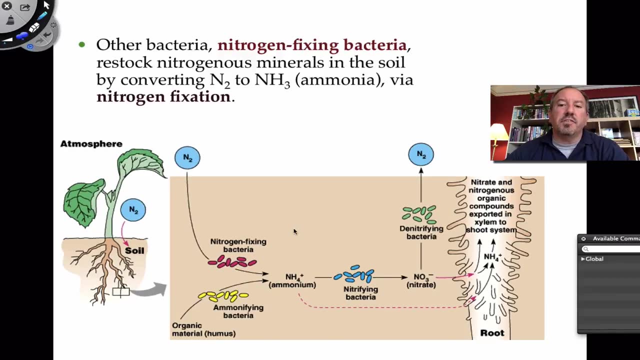 There's nitrogen gas coming out of the soil. Nitrogen gas, How's that? Denitrifying bacteria are bringing it back into the atmosphere to complete the cycle. Okay, So here's the emphasis. now, This nitrogen-fixing bacteria are so critical, because this is literally the bacteria that pull the gas out of the air. 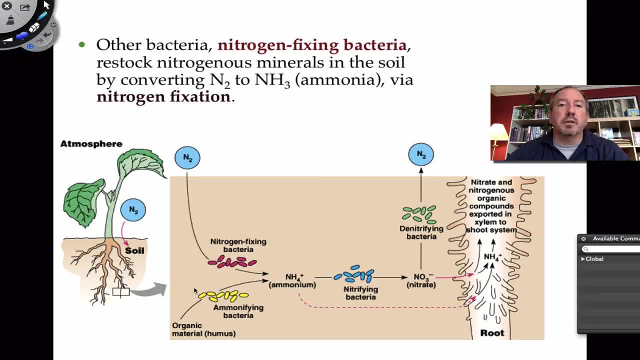 Now the ammonifying bacteria are also critical because they're helping to break down detritus. But nitrifying, Nitrogen-fixing, Nitrifying bacteria are literally pulling nitrogen gas out of the air, producing ammonium. They're really important. 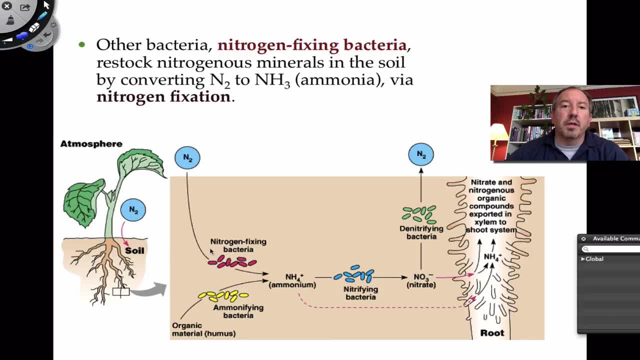 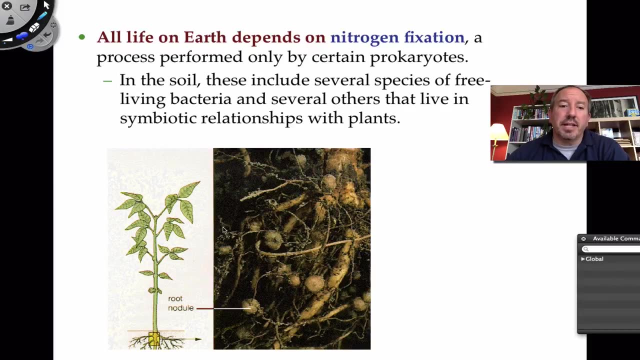 They're either free-living in the soil, So, in other words, soil on its own can actually become more fertile if you have a lot of nitrogen-fixing bacteria, And then this is what's really, really cool. We've discovered that some plants, some plants, actually have these nitrogen-fixing bacteria living in the roots. 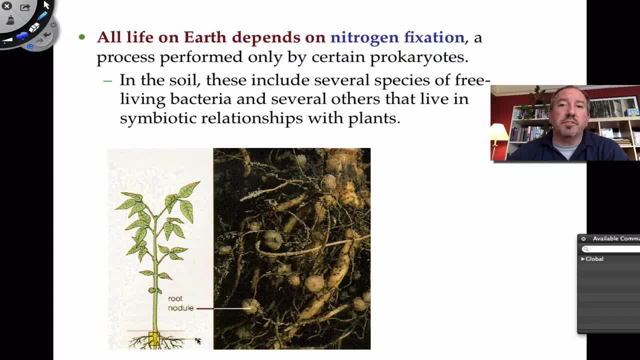 So there's a symbiotic relationship between these nitrogen-fixing bacteria and certain plants And the class of plants called legumes. So things like alfalfa and clover and peanuts all have this bacteria. And again, these are not individual bacterias, but these are these root nodules. 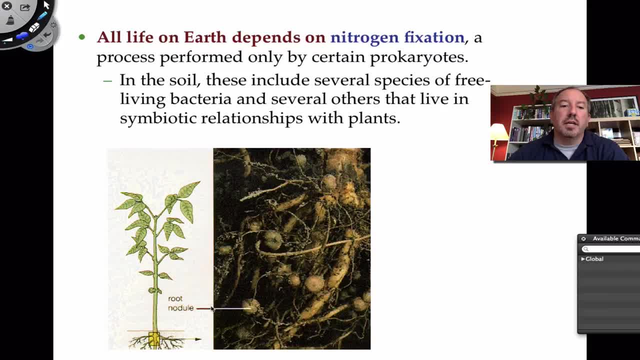 And there's like colonies of bacteria living there. So how about this? If you were to plant that crop, Like if you were to plant Alfalfa, if you will, in between, when you're planting corn, the alfalfa, since it has a lot of nitrogen-fixing bacteria. 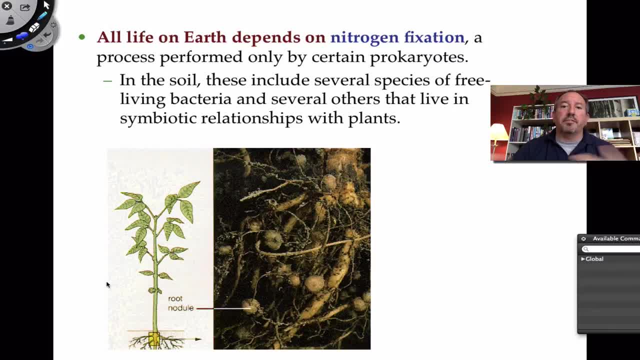 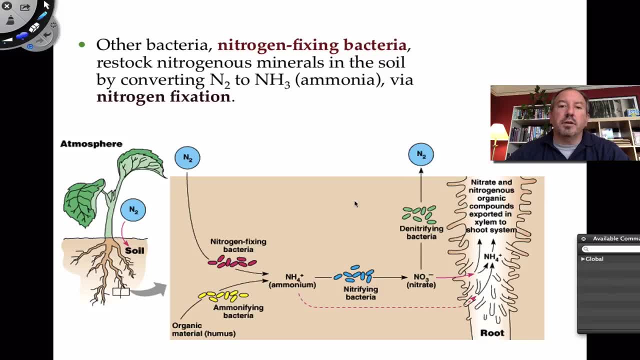 will draw a lot of nitrogen out of the air and will actually fertilize the soil for you, naturally, Because if you wanted to put artificial soil, Say you wanted to make your garden grow really efficiently, Maybe you'll add some like Miracle-Gro or something like that. that's a name brand, Miracle-Gro. 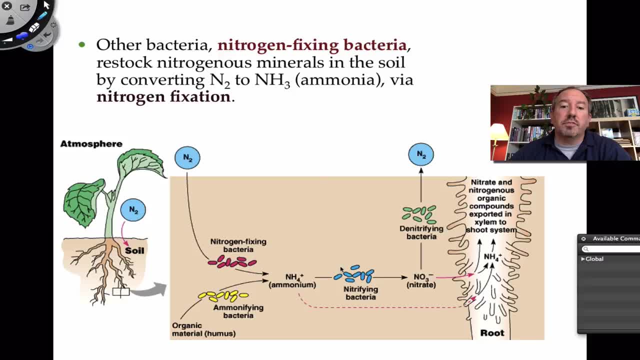 What is Miracle-Gro? What does Miracle-Gro have in it? It has nitrates, nitrites and ammonium, And it also probably has a little bit of phosphorus too And some potassium, But basically it has nitrogen in it. 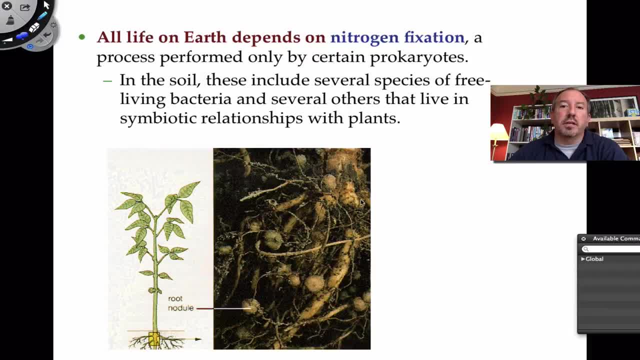 And it's like: well, if you don't want to add fertilizer, what you could do is These nitrogen-fixing bacteria will help fertilize the soil as well, And so I mentioned symbiosis. It's mutual, because what do the bacteria get? 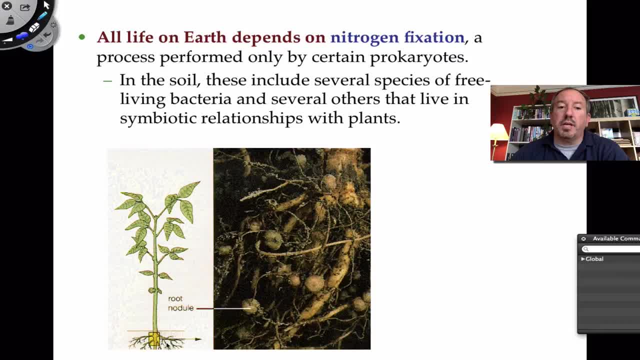 Well, they get sugar from the plant through photosynthesis. So it's pretty neat. This plant kind of comes along with its own. This plant kind of comes along with its own. This plant kind of comes along with its own bacteria to help fertilize the soil. 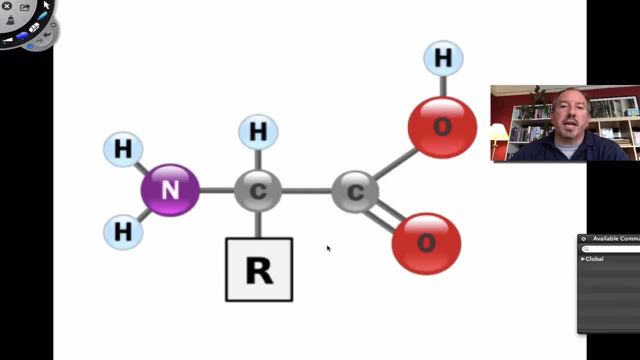 Pretty awesome, And so here's a picture of an amino acid, And again, this is critical. There'll be a future discussion where I talk about the biochemistry of these molecules, But without that purple nitrogen coming from the soil, plants are not going to be able to make amino acids. 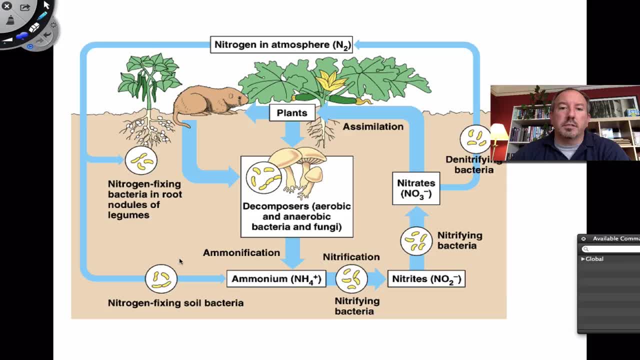 And they're not going to be able to make DNA or RNA, And so it's rather critical. So this diagram summarizes the nitrogen cycle, So let me go over it kind of quickly, because we've been talking about this. So let me just sort of trace the nitrogen this way. 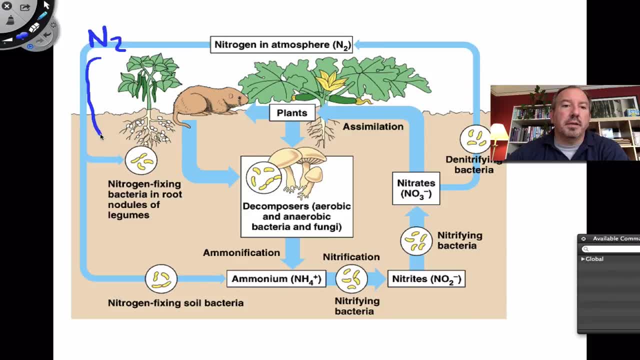 So nitrogen gas in the air can come in, and it can be picked up by nitrogen-fixing bacteria if it happens to be on some peas and beans, or also legumes, And so those will produce ammonium as well. So nitrogen-fixing either on plants or free-living in the soil. 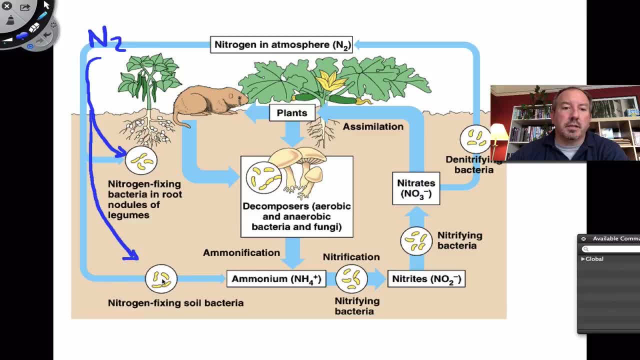 nitrogen-fixing. this is both nitrogen-fixing bacteria, nitrogen-fixing bacteria. nitrogen-fixing will produce ammonium. Now there's the ammonifying bacteria that I mentioned before. When everything dies like here's some zucchini, here's a zucchini blossom. 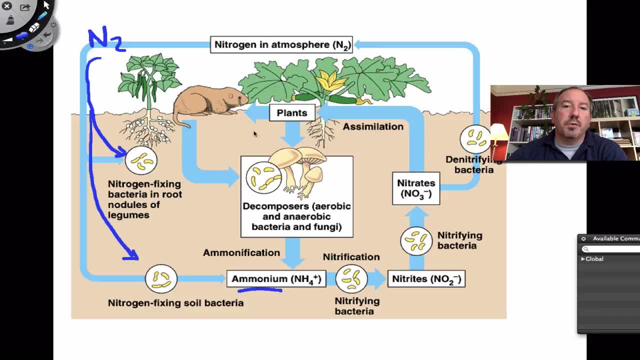 It's very delicious if you've ever had that to eat. So when everything dies- all the plants, animals, everything's dying bacteria, the ammonifying bacteria are breaking it down into guess what ammonium. Then you have the nitrifying bacteria that are turning it. 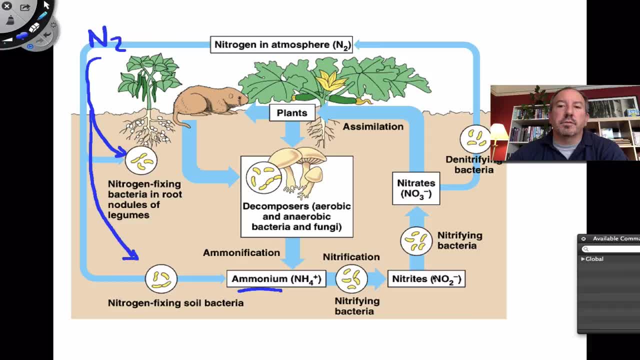 into ammonium, Nitrates and nitrites, which are preferable to be assimilated by plants. So the nitrates, nitrites and ammonium can go into plants. And what do they do with them? They make the amino acids which are needed to produce proteins. 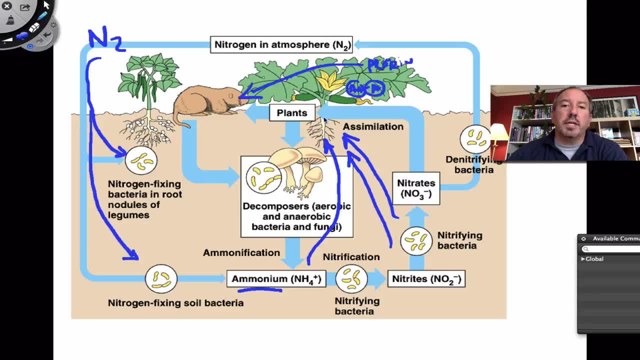 Okay, And then who's eating the protein? We are eating the protein. So how do we get nitrogen? Eating plants or eating animals, Depends on how we're where we are in the trophic level, And then, finally, denitrifying bacteria return the nitrates back into the atmosphere. 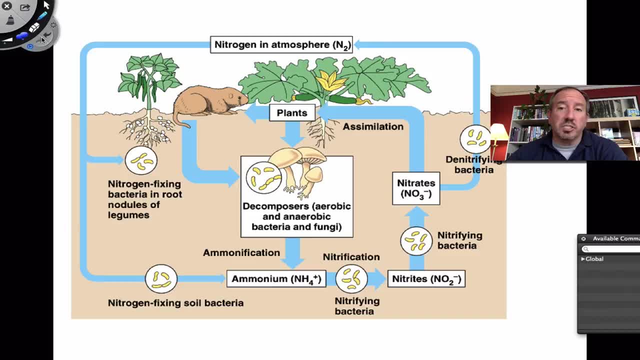 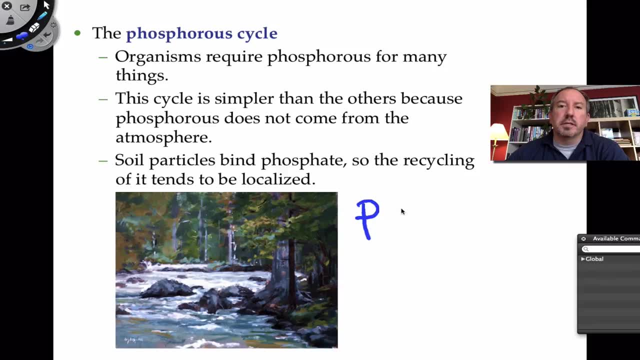 And then you get the cycle going around. So the nitrogen cycle, Now the phosphorous cycle. the element phosphorous is very important as well, And you're like: well, why is that very important? It's important because it's also found in DNA. 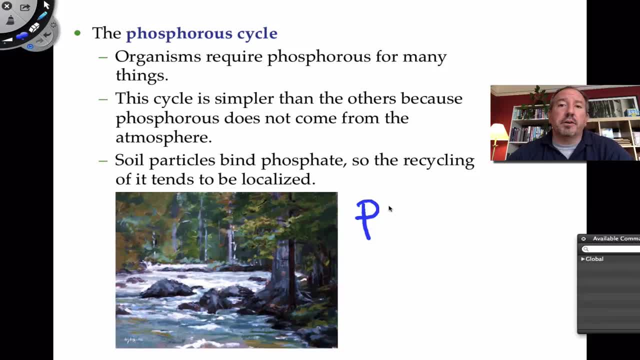 It's also found in a structure in the cell membrane and all of our cells called the phospholipid. It's also found in a very important energy molecule called adenosine triphosphate, And I can go further with that, but this is say that it's very important. 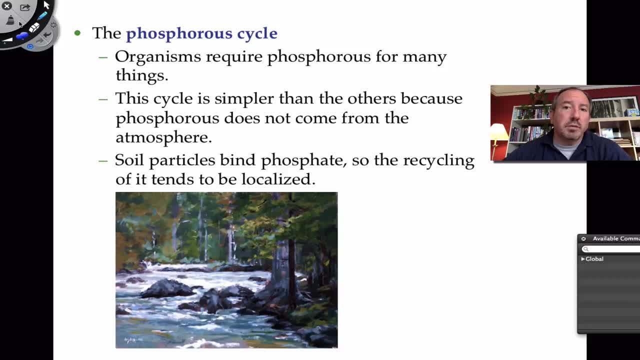 The thing about the phosphorous cycle is that it's a little bit more easy going because there's no gas form of phosphorous. And if there's no gaseous form of phosphorous it doesn't mean that it's going up into the air. 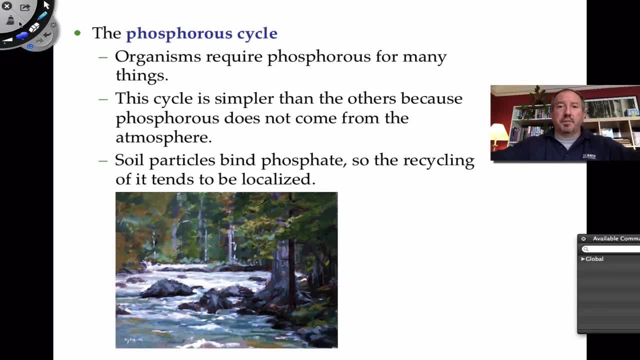 Like. in other words, the soil isn't releasing it. The soil is not releasing. It's not blowing all over the place, which means that it's more of a local cycle. So we have phosphorous Plants have phosphorous Animals have phosphorous. 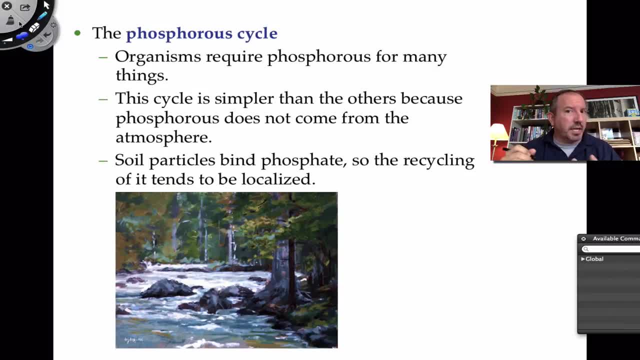 And so we're kind of local. especially a plant, a tree. So when the tree has it and dies it's going to go right back into the soil and it's going to be picked up by the future plants. So it's kind of a local cycle. 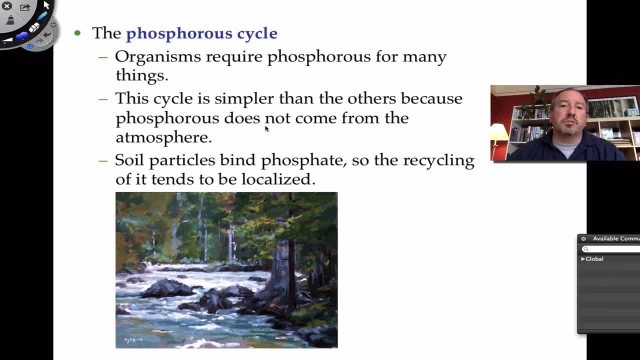 So, as I was mentioning, organisms need phosphorous to survive And it's a little bit easier going because there's no atmospheric compound And, as it turns out, it has a lot to do with the soil, because phosphorous is in the soil. 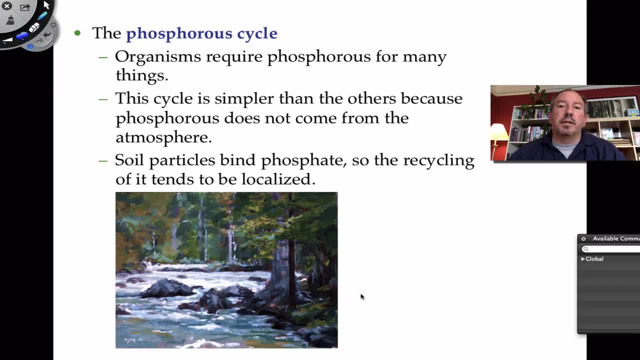 Now it's usually not limited in the soil. Now, of course, if you're growing lots of crops, they're going to need a lot of phosphorous. Where it is limited is in the water, And actually that's a good thing. 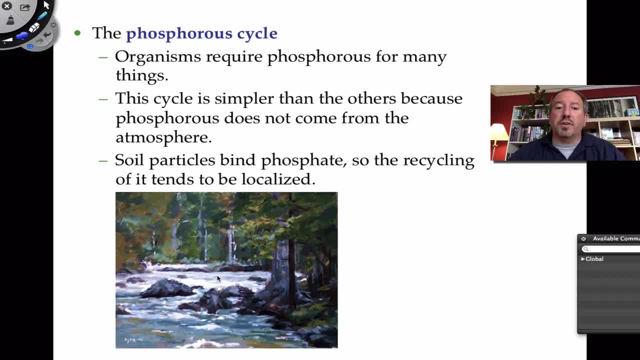 We had talked about this once before. If you looked at a previous video, sometimes too much phosphorous in the river will cause algae to grow. It's like, yeah, phosphorous, And then you don't want that, because then it dies and it depletes the water. 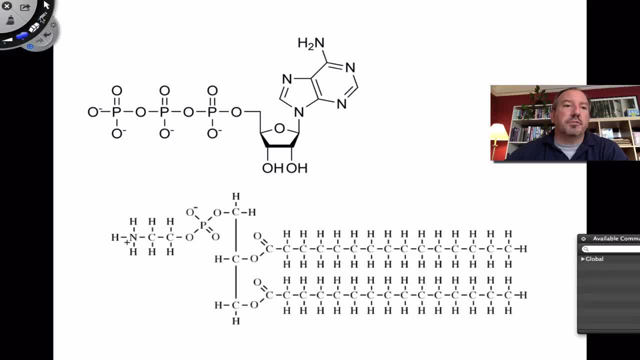 And so I was mentioning a chemical called adenosine triphosphate, And so this is what it is: adenosine triphosphate, ATP- There's the phosphate, There's the phosphate And there's the phosphate. So in order to produce this molecule, you need to get phosphorous. 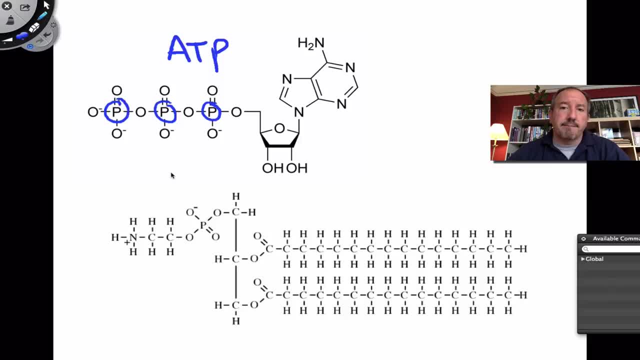 Where do we get phosphorous? Well, we get it simply by eating. Animals get it from eating. Where do plants get it? The soil, And so this is a structure called a phospholipid. It's a little bit like that. 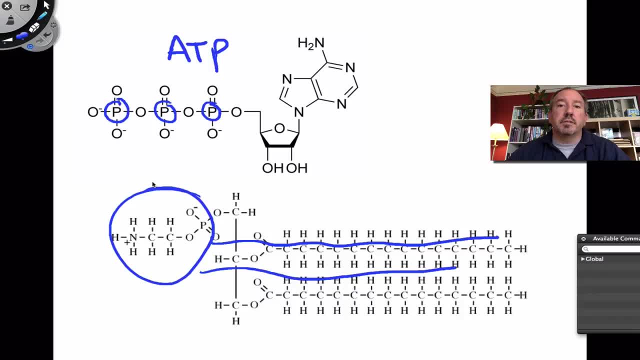 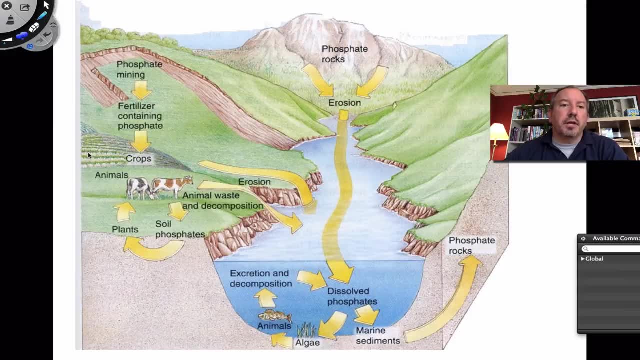 There's the phosphorous, And then there's these two tails that come off of this. This is a component of the cell membrane, So plants need to get phosphorous from the soil, And so here's some crops They're growing. They're loving it. 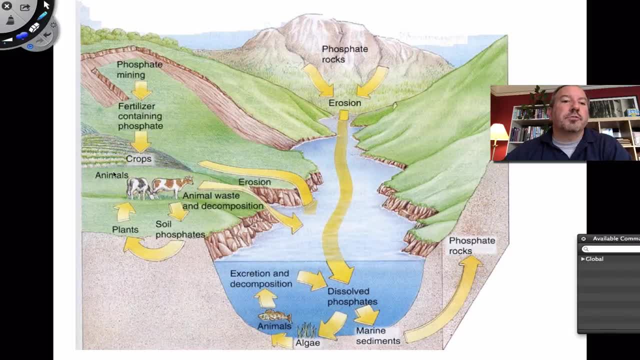 They're getting phosphorous from the soil. How'd the phosphorous get into the soil? Well, you know, it's in rock as well, And then rock can be broken down through just water. Weathering processes were physical, And then, through rain and erosion, it can actually go into water. 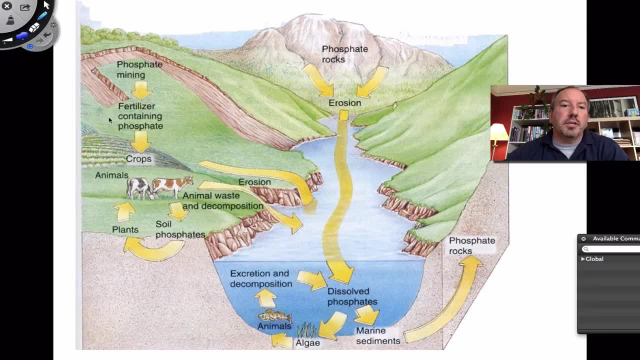 But basically it's in the soil And, as it turns out, we could use it as fertilizer- although we want to not use too much of it- And then again it helps plants to grow. And then where do animals get phosphorous? from eating the plants? 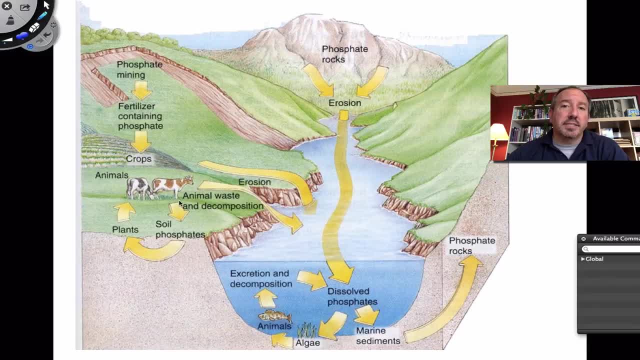 And so when a plant and animal dies, it's simply broken down by bacteria. I won't go into the metabolism of that, I'll just keep it simple. The phosphorous is then broken down and it goes into the soil. So how about this? 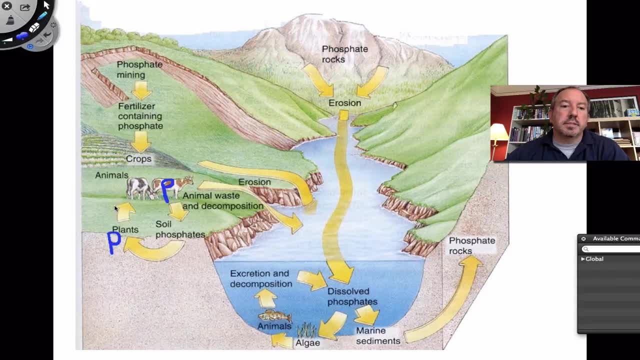 Phosphorous is in the soil, Then it goes into the plants, And then it goes into the animal, And then when the animal dies, it goes back into the soil, So it's kind of a local cycle. It's really important though. 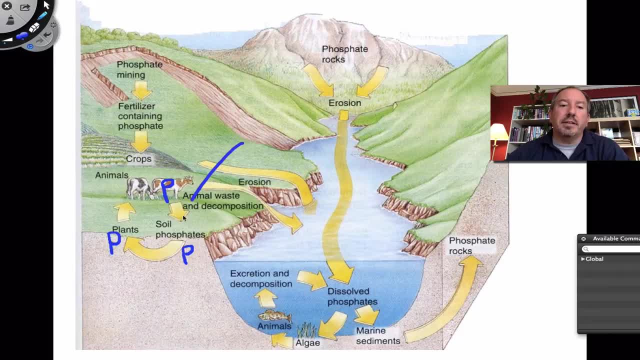 And again, just to emphasize this you don't want to add. you know it's like humans have a tendency to be kind of greedy And sometimes selfish and short-sighted. sorry, But we add way too much phosphorous to our soil. 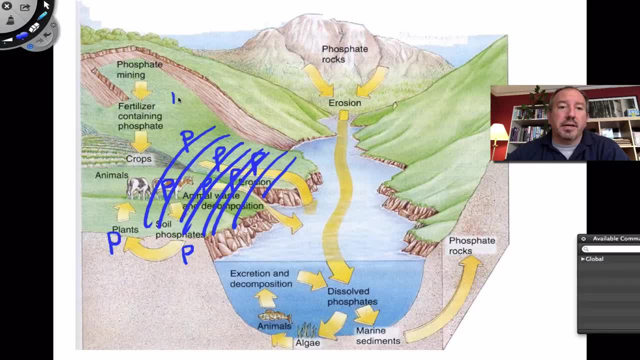 because we want our crops to grow. And then we're like: well, when it rains again, all that runoff of phosphorous into the water and all the algae is thinking, oh, this is awesome, I love all this phosphorous. 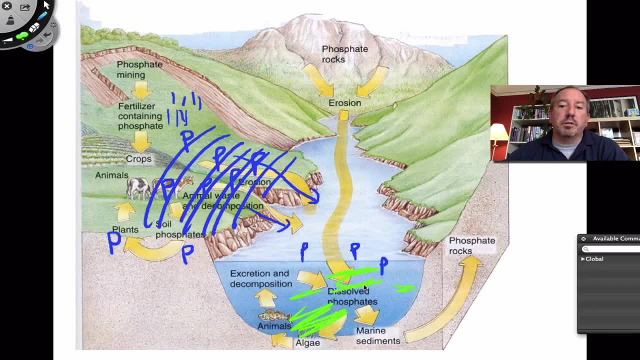 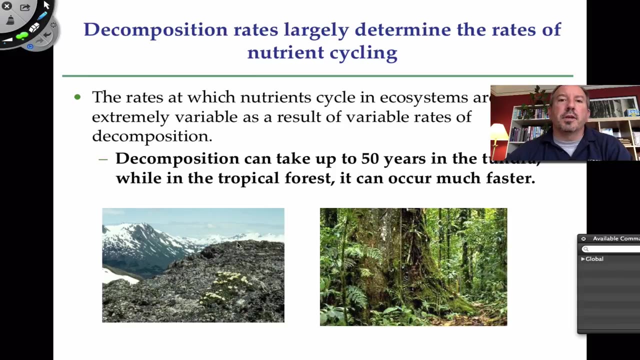 I will grow like this and form big algae blooms, And then what? Then the algae dies and the decomposers will consume all of the oxygen And therefore the water is injured as a result of too much phosphorous in there. And so I just wanted to say that decomposition. 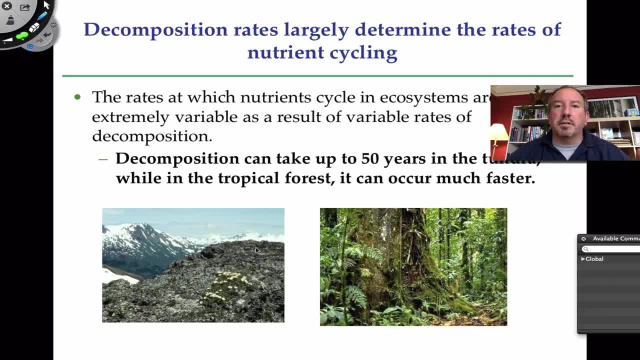 is really what we're talking about in the carbon cycle and what we're talking about in the nitrogen cycle and phosphorous. It's these decomposers. Again, the smallest microbes are of the most importance, And I think that is something that needs. 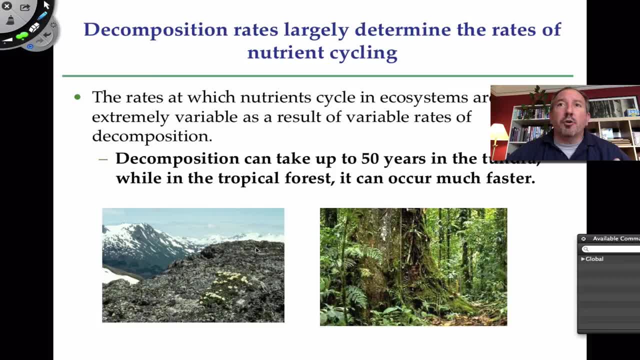 needs to be considered. And so, when we're talking about how quickly does this chemical cycling take place? Well, it depends on where you are, Like, for example, if you're here in the tropical rainforest and it's very moist and there's a lot of warm temperature. 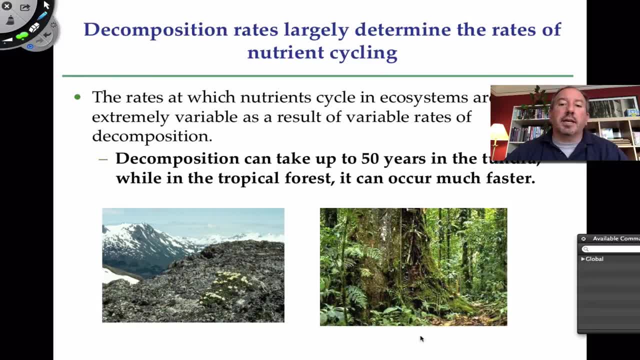 decomposition occurs very quickly, So the nutrient cycling is boom, boom, boom. But if you're up here in the tundra where it's like a freezer, it can be really, really slow, And so the recycling happens very, very slow. 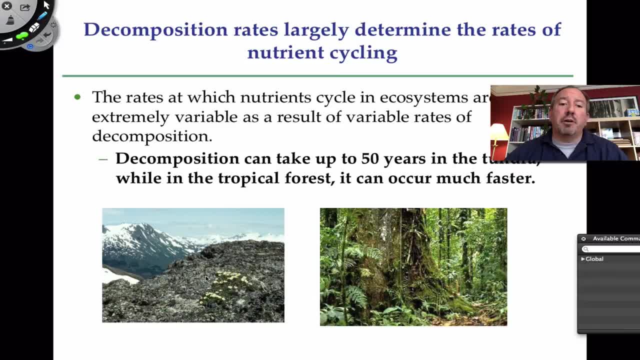 And so that's a factor when you're looking at biodiversity. If the nutrients aren't cycling very quickly, then you're not going to be able to support a lot of vegetation and therefore not a lot of trophic levels, And so that's of consideration. 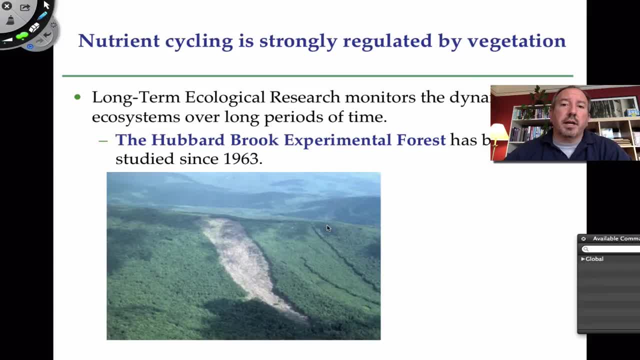 And so, finally, in this discussion of biogeochemical cycling, I have to mention one of the classic ecological experiments of all time, And it was conducted in the state of New Hampshire, in a region on a mountain slope called a watershed. Now, a watershed is basically like this: 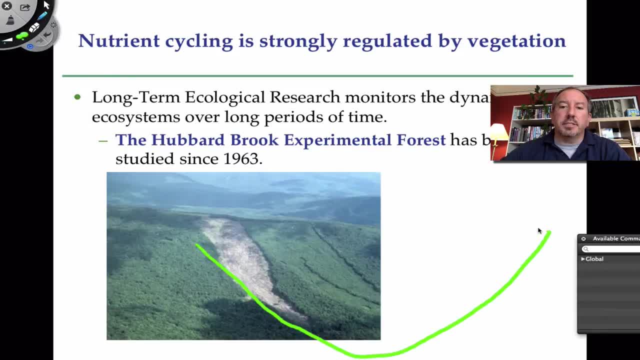 If you have again a valley like this, And so these are trees And a watershed, is this valley, And when it rains, the water runs down on both sides of the valley And it basically goes down into a river. This is what we mean. 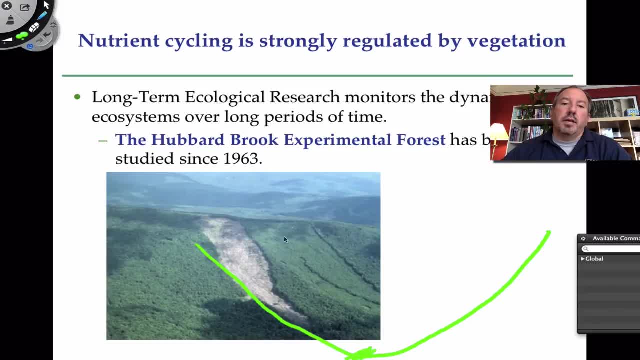 This is what we mean by a watershed, And so in terms of logging, like when you want to cut down some trees, it's very difficult to cut down just a couple of trees and then move over here and cut down a couple trees. It's much easier to sort of clear, cut a big patch. 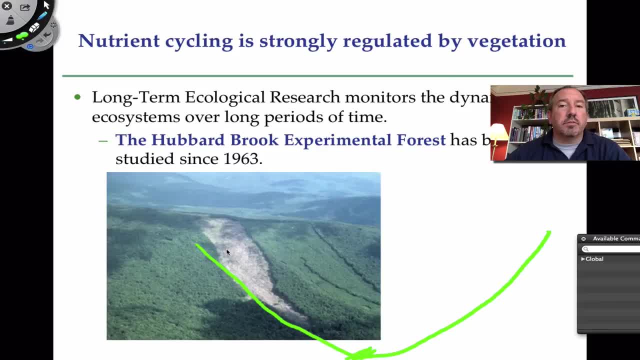 while you have the trucks there and hauling it all out. It's tough work, And so ecologists always wondered what is the effect of the loss of vegetation, In other words the forests, on nutrient cycling? And so what they did is they went out. 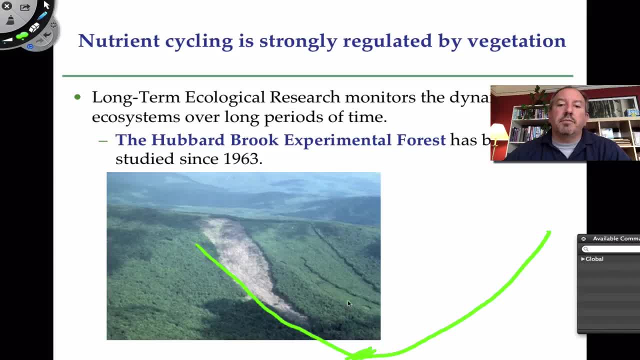 and they decided to do a long-term research study of this one little brook, this one little river in an area and it was called the Hubbard Brook. So the Hubbard Brook experiment has been studied since 1963. So in 50 years the data has been collected here. 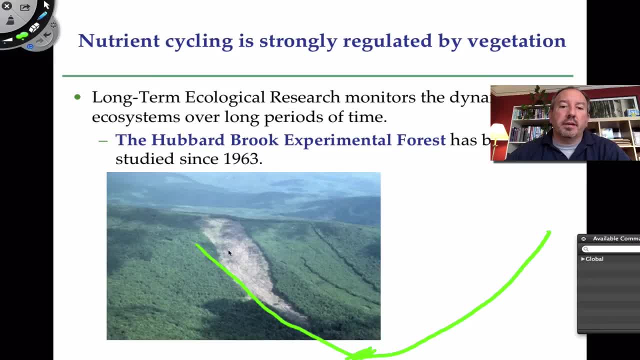 So what's interesting is that on one side over here, an area was clear cut, So the trees were removed. So take in all the stuff that we've been talking about and how vegetation trees take in nutrients from the soil. Okay, what's going to happen if you remove and clear cut an area? 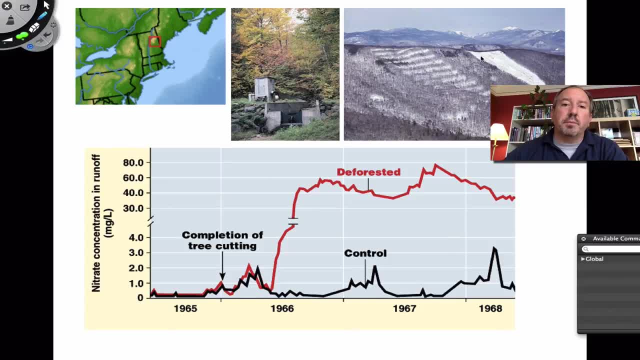 This is the Hubbard Brook area in the wintertime. You can see how it's white. up here It's snowing Now. when the water runs down the mountain, it's not just pure water. It's carrying a lot of nutrient like nitrogen, phosphorus. 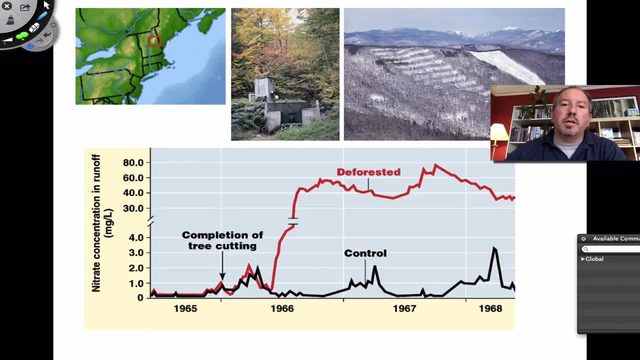 and what have you? And at the brook, this is the place where the water was sampled by the researchers. And then this is where the Hubbard Brook is, in New Hampshire, And so check this out, We're looking at the levels of nitrogen. 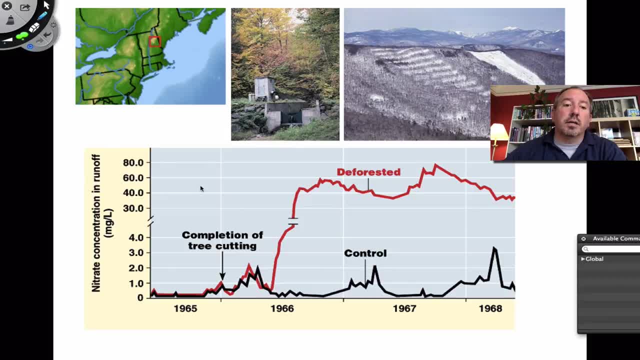 what is it? nitrate in the water at Hubbard Brook. Look at this here. Look how the numbers go from one all the way up to 80.. It's so large it has to be broken up here. So in other words, 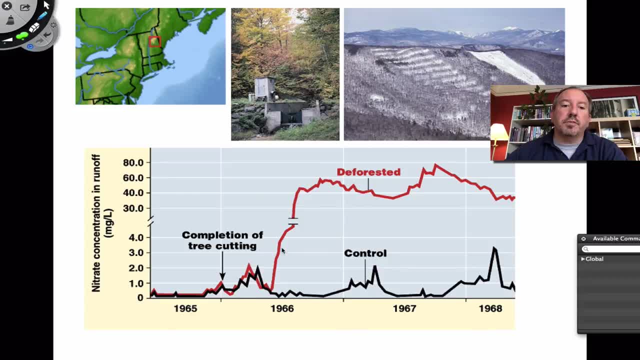 when the forest is intact, when you don't cut down the trees, the level of nitrogen in the water in the brook is relatively low, and it remains relatively low. Now why is that? It's because the trees themselves are either holding on to the nitrogen or the root system is taking the nitrogen up, and when it rains, the nitrogen is remaining in the soil because of all the trees. 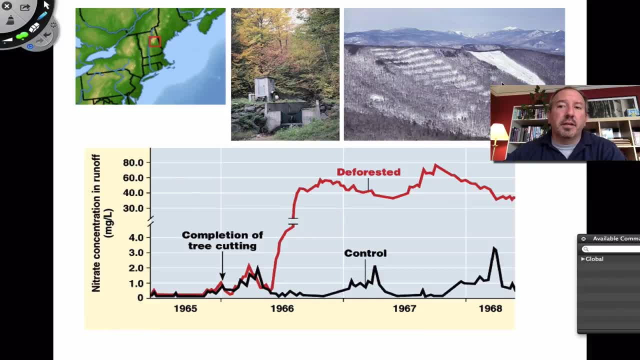 If you cut down the forest like this, what's going to happen is there's no more vegetation, And so, when it rains, all those nitrogen compounds are going to run off and go into the brook. So look at the levels of nitrogen in the deforested area. 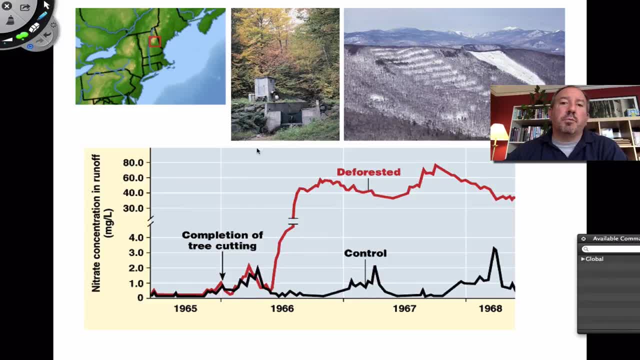 Now this is devastating because all that nitrogen that goes into the water, what's that going to do for the algae? It's going to love it, It's going to grow, grow, grow. it's going to deplete the oxygen and it's it's going to basically kill everything down below. 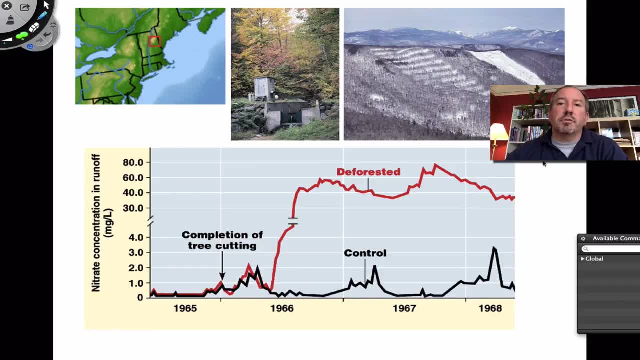 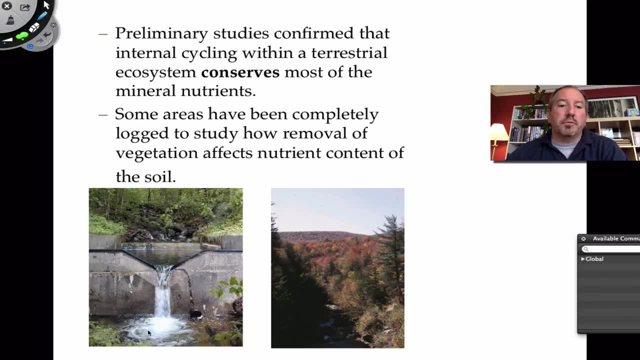 And so how do you like this? The river systems are destroyed, The fish are destroyed Because of all the nutrient runoff, And so, as it turns out, this is a close up of where the water was studied, where those numbers were picked up. 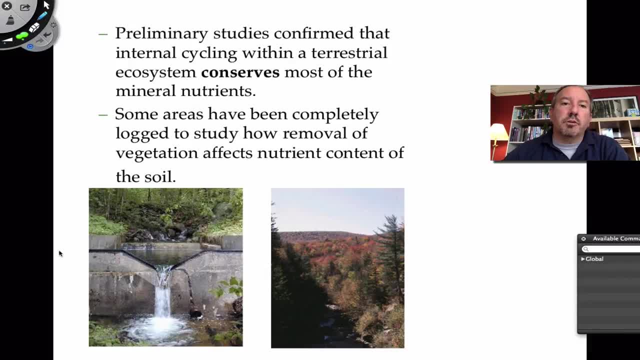 And so preliminary studies confirm that there is an internal cycling in land ecosystems that can serve most of the mineral nutrients- This is what we're talking about- the geochemical, biogeochemical cycles- And so that when you log an area, you can affect the nutrient content in the soil. 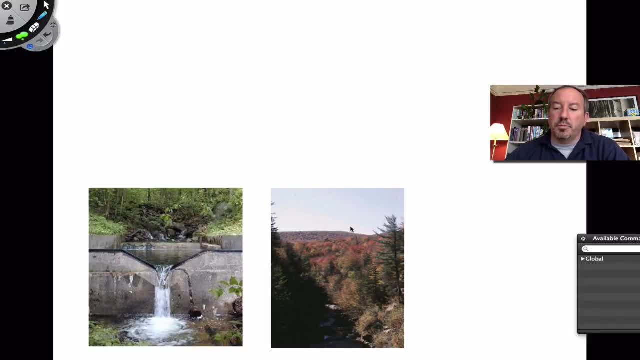 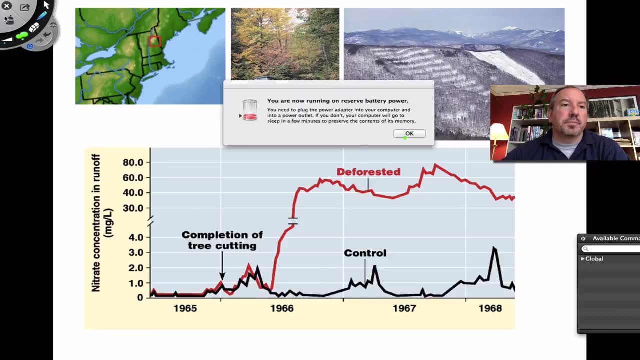 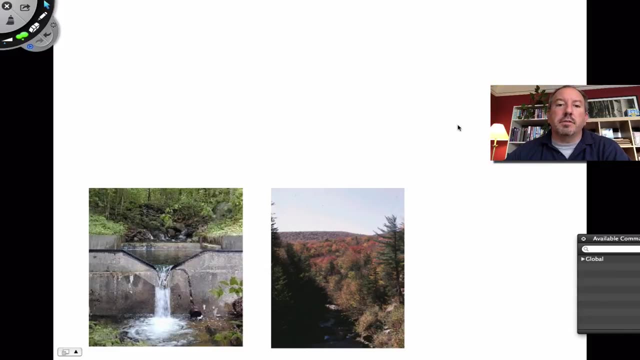 And so a loggers, We'll say, Well, I'm just going to, you know, replant the trees, settle down. And it's like, well, you're not just going to replant the trees, You're not just going to replant the trees, because the soil quality itself is going to be depleted, because a lot of it's going to run off into the Hubbard brook. 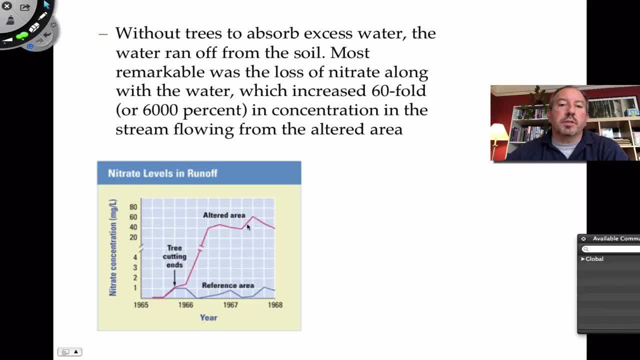 And so again, here's another look at how much nitrogen was released from the area Once the forest was cut down: sixty fold increase, which is six thousand percent in concentration. So there is a continual increase in the amount of nitrogen released out of this area. 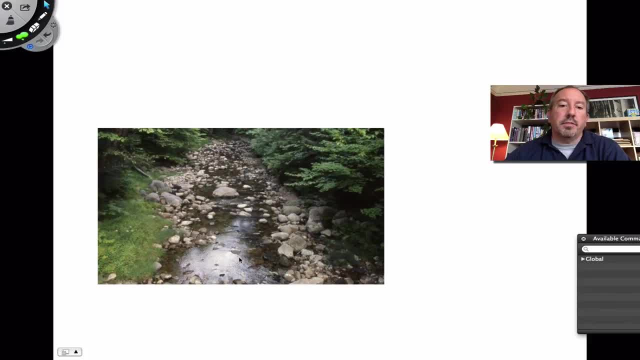 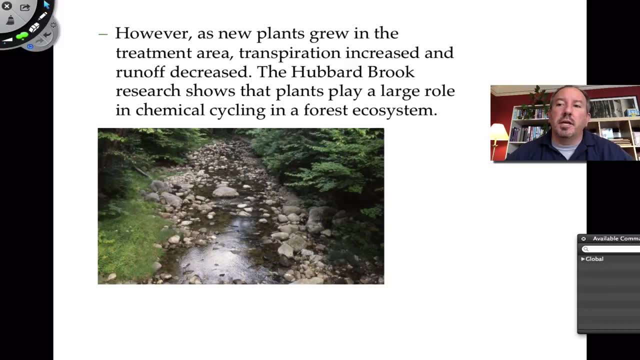 So again, here's another look at how much nitrogen was released from the area once the forest was cut down in the stream, And so the river systems are possibly destroyed, And so this is a real important thing. So just to bring this close to home, in California we talk about the logging of 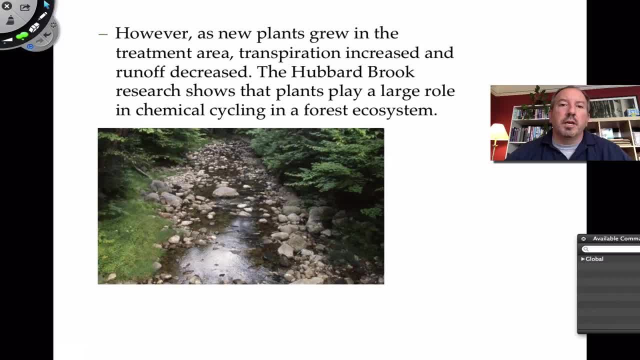 redwood forests And we're like: well, those are really precious And well, it's not just the loss of the trees in the forest ecosystem, but the water system is also compromised as a result of this massive logging. So all these things need to be taken into consideration because in an ecosystem,